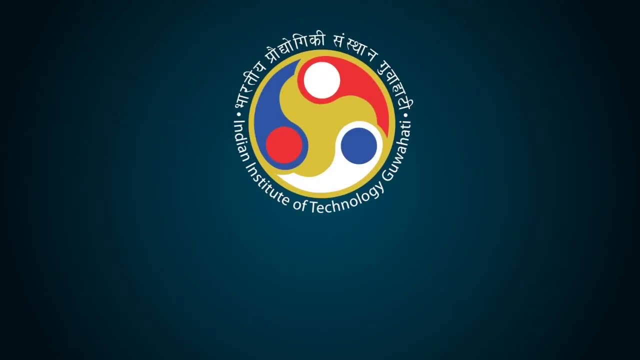 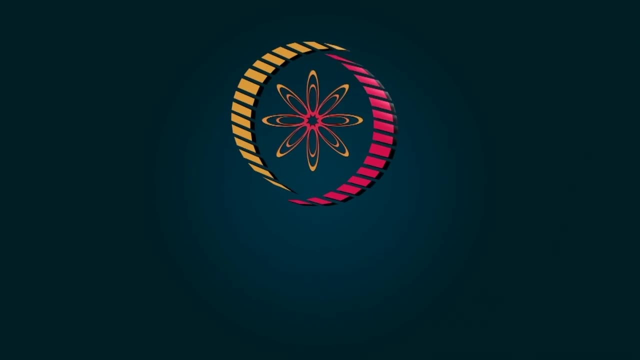 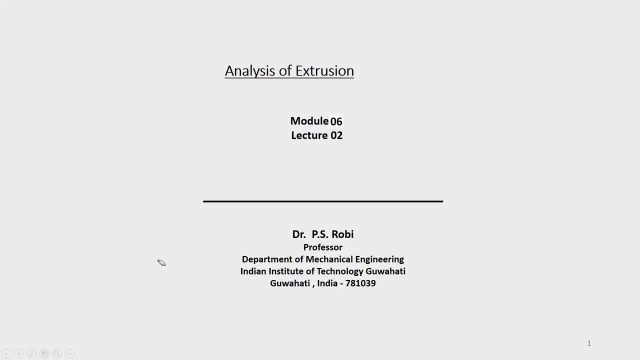 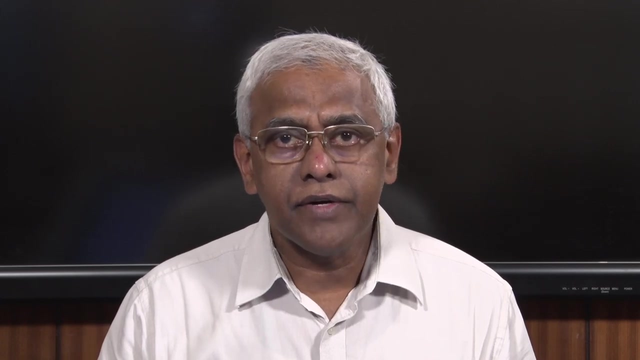 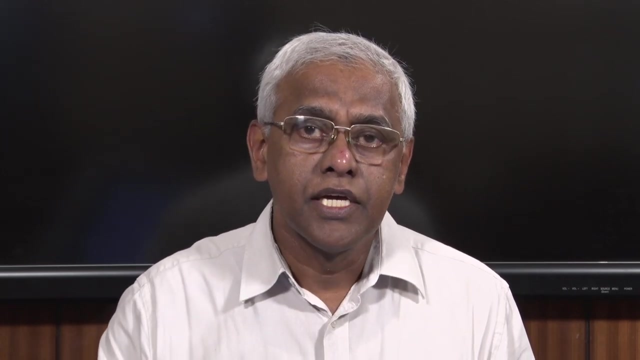 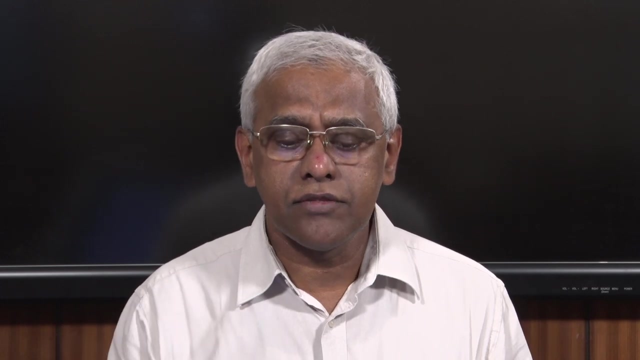 In this lecture we will be discussing about the analysis of extrusion. That means to determine what is the load necessary for the extrusion. for an extrusion process It may be cold deformation or cold extrusion, or it may be hot extrusion, but the analysis is more or less similar. So when you wanted, 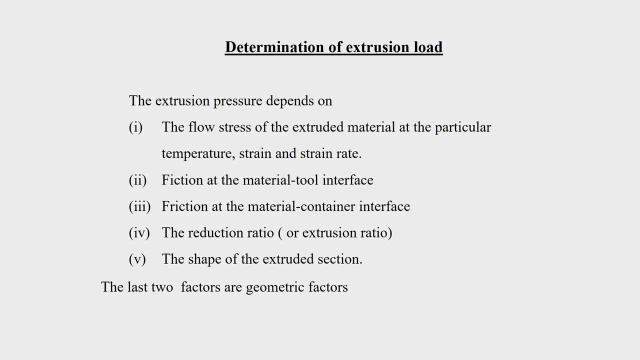 to find out the determine the extrusion load. what is done is calculate the extrusion pressure and then you multiply it. Multiply by the cross sectional area at the inlet side, that is, at the container side, Cross sectional area of the inside, cross sectional area of the container. so that is. 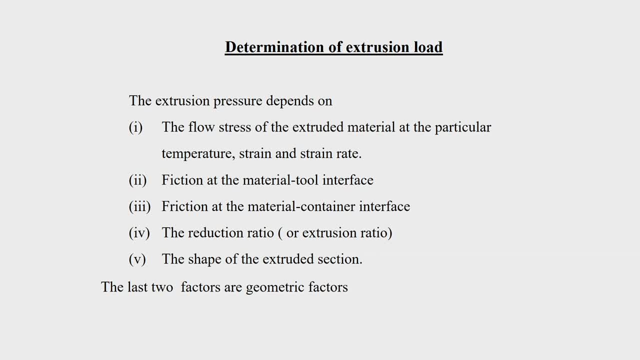 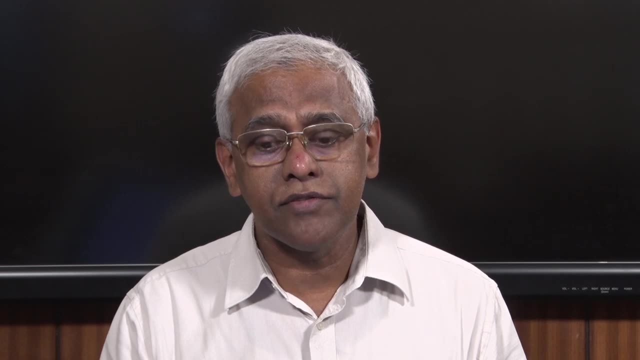 what we will do, that The extrusion pressure, or the pressure required for extrusion process. that depends upon the flow stress of the extruded material and the flow stress. you know that that also, in turn, depends upon the temperature of deformation, the strain and the strain. 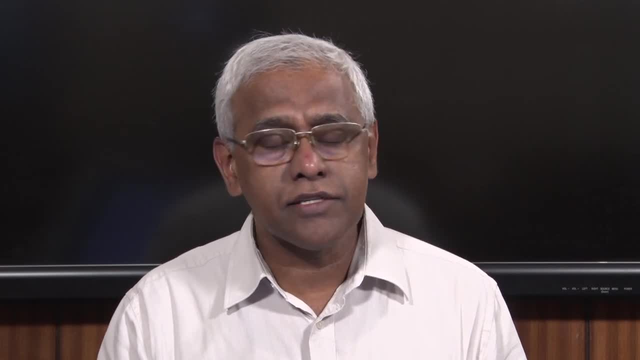 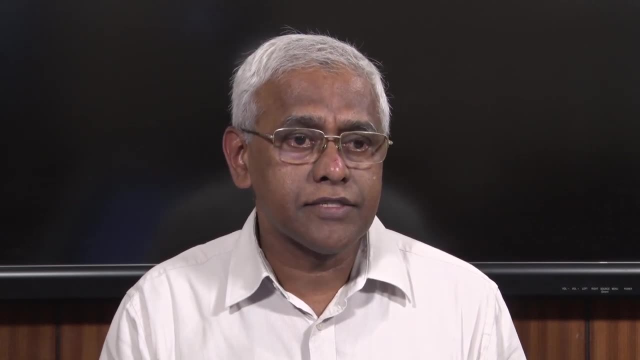 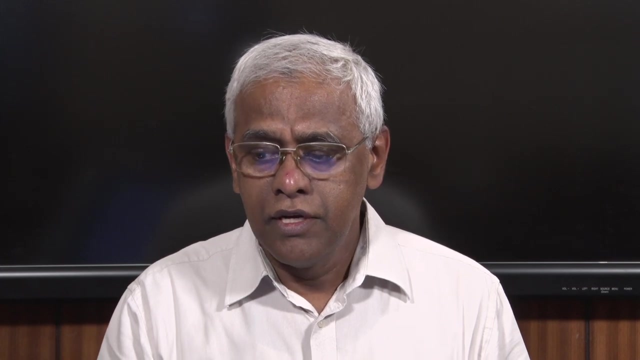 rate, Because if it is at a higher temperature, naturally the flow stress will be lower, but there is a strong dependency on the strain rate, because strain rate sensitivity comes into picture. So, though, flow stress will be lower, but that is there, And then it also. depends on the friction. 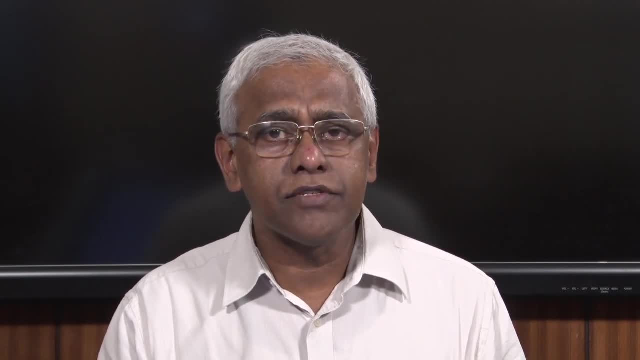 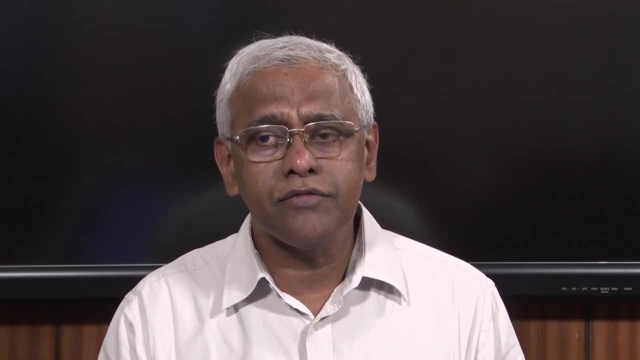 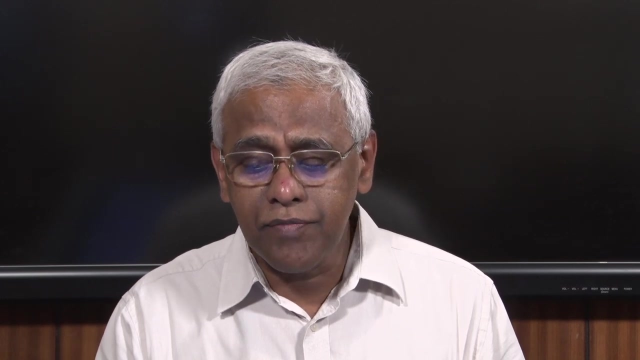 So the ingot or billet which is to be used is cylindrical in shape, and then, okay, this material will be deforming in the inside once it reaches the deformation zone, that means where the die comes into picture. So the it depends upon the material tool interface: friction, okay, or friction at the 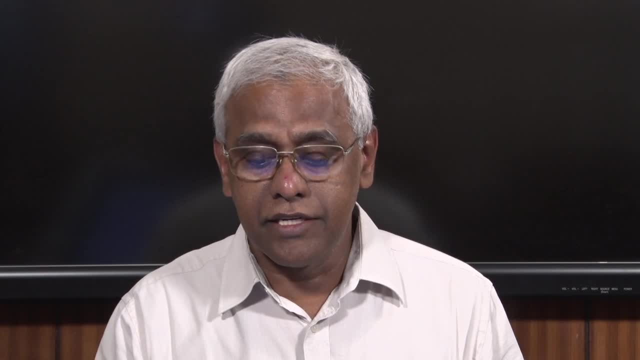 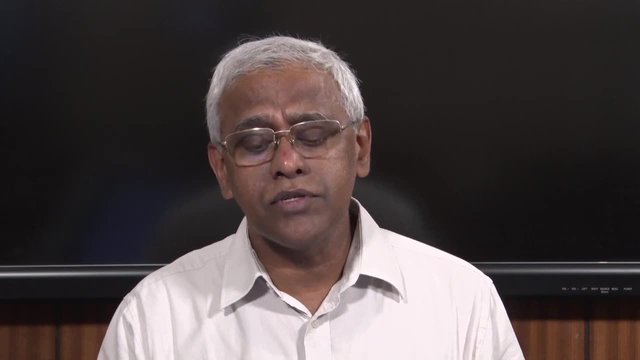 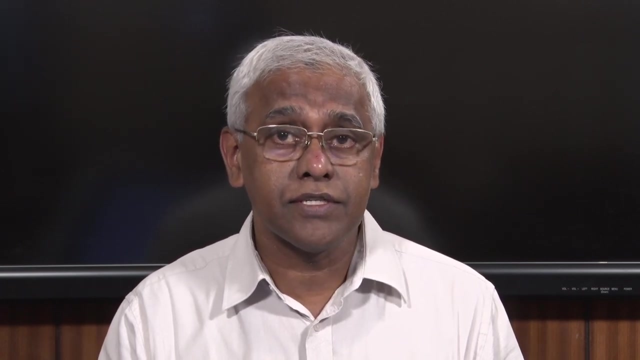 material tool interface or material die interface. and another thing is there: if it is a forward extrusion, then you will find that there is going to be large amount of friction at the work piece and the cylinder or the container, because this part we have discussed in the 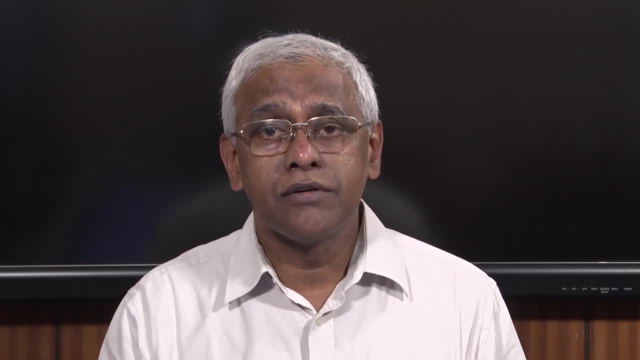 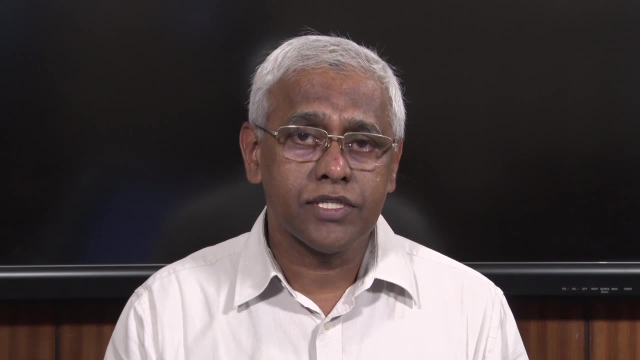 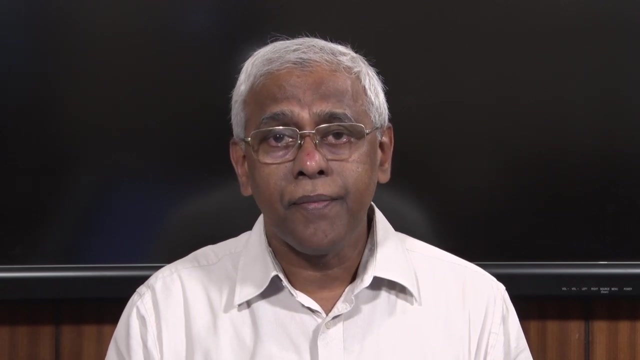 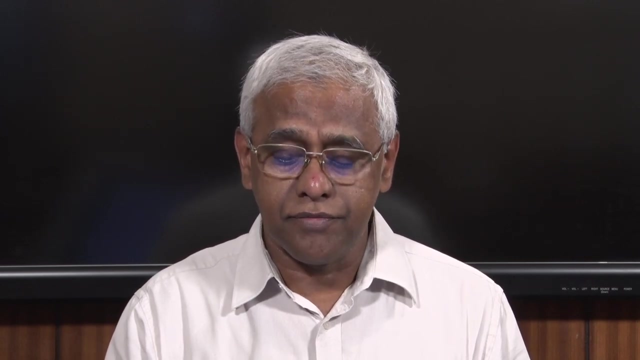 last class, and we also found out how the load versus ram displacement will look like for both forward extrusion, backward extrusion and hydrostatic extrusion, all those things we have discussed. So the friction between the Cylinder and the billet, that also comes into picture. then what is the amount of reduction? 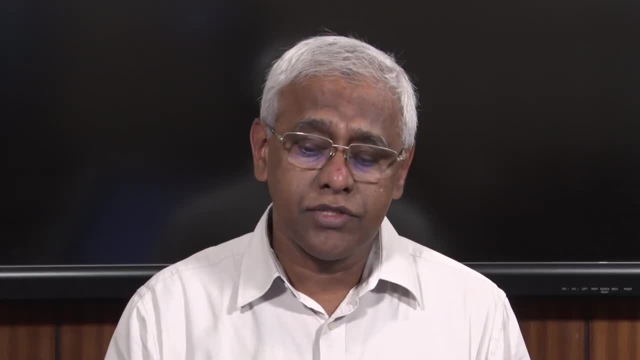 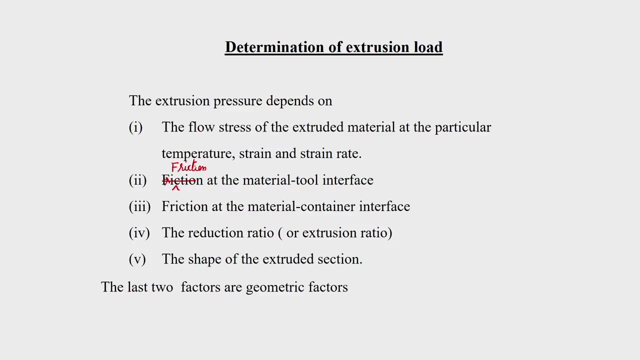 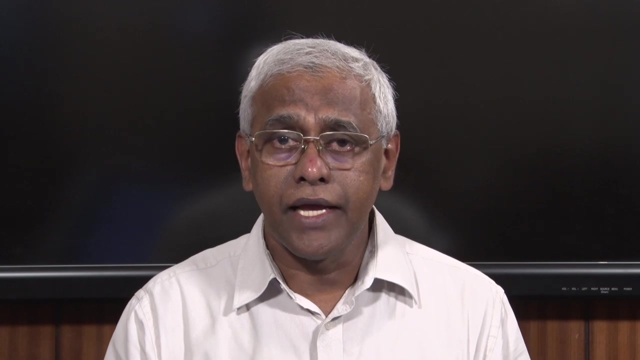 or normally in extrusion, if we do not use the word extrusion reduction ratio, rather we use the word extrusion ratio. okay So, but ultimately these two are related. also we can directly, so in a way we can say that what is the reduction ratio? so extrusion pressure depends upon higher the reduction ratio, or 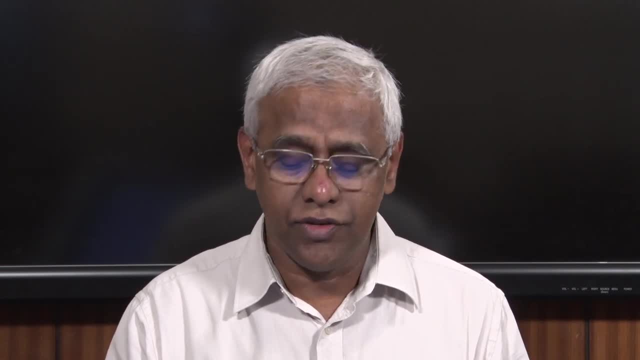 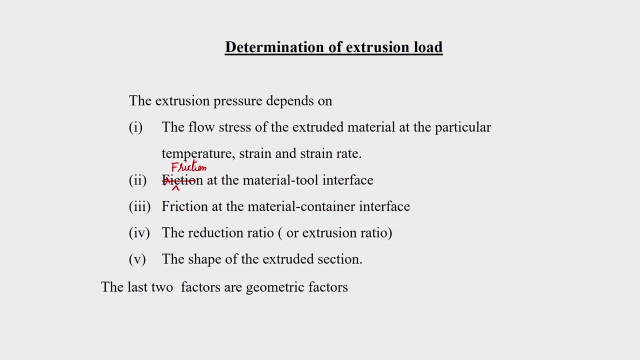 the higher the reduction, the higher will be the extrusion pressure which is required. okay, because one is internal shearing. everything will come into picture then: the shape of the extruded section. that is very important. see, if it is a cylindrical to cylindrical piece, it is very simple. okay, analysis also becomes easy. cylindrical to square also, it is a problem. 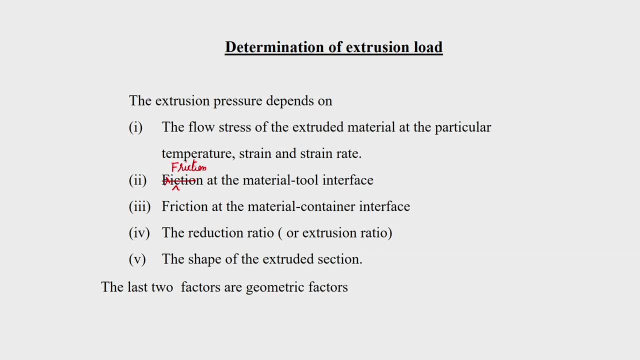 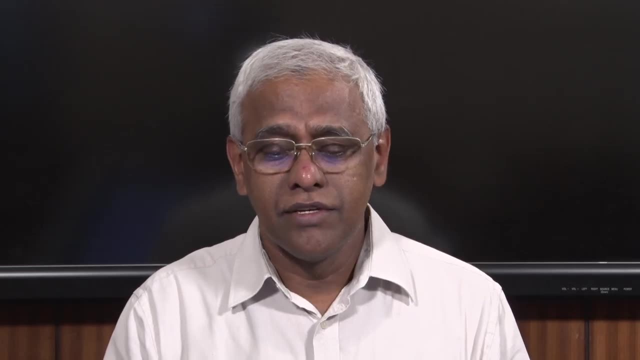 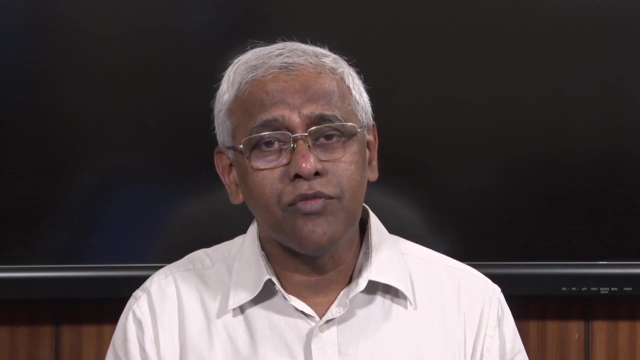 but most of the case, especially non-ferrous materials and, like aluminum, magnesium they wanted. So it is a very specific section, cross sectional area, which is very complicated, so and the level of complexity when it increases, the extrusion pressure also increases. Now, another factor is that how many are there, for sometimes you may have multiple number. 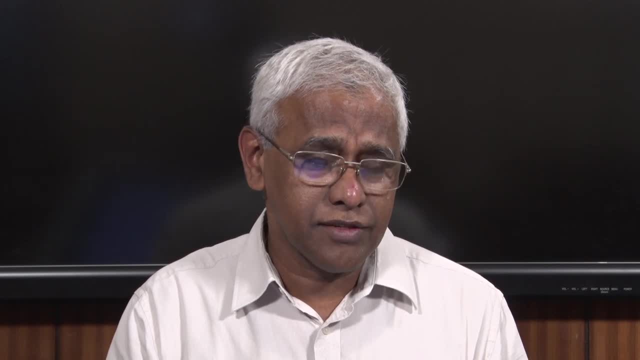 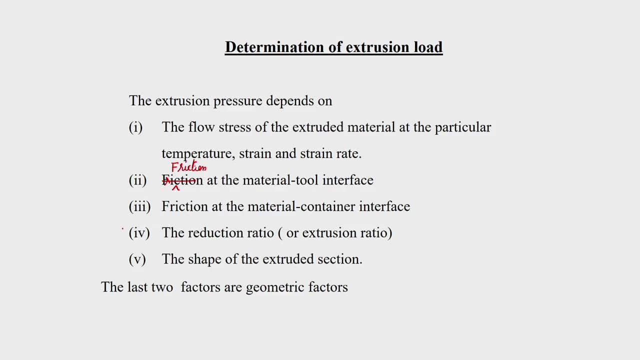 of extrusion inside a die itself. that also complicates the thing, but the production is much faster, so those type things comes into picture. So the last two, These, These are the factors which are mainly due to the geometry- okay, the other the frictional. 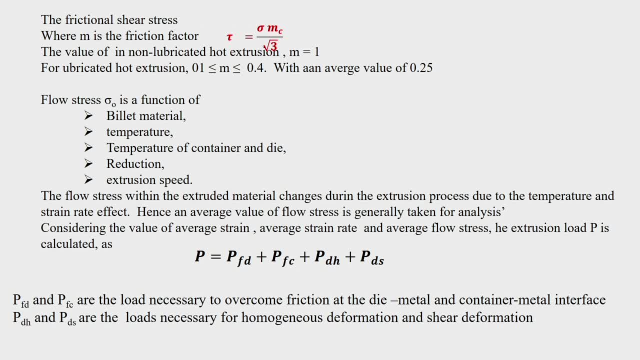 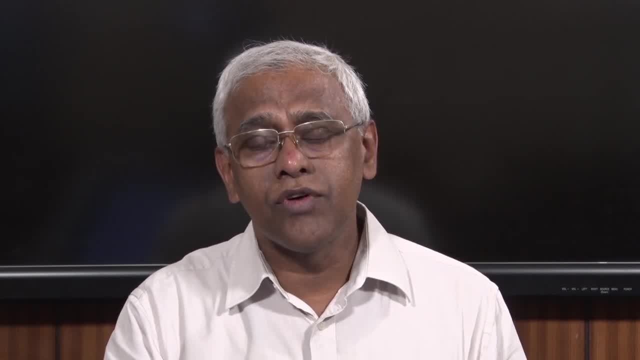 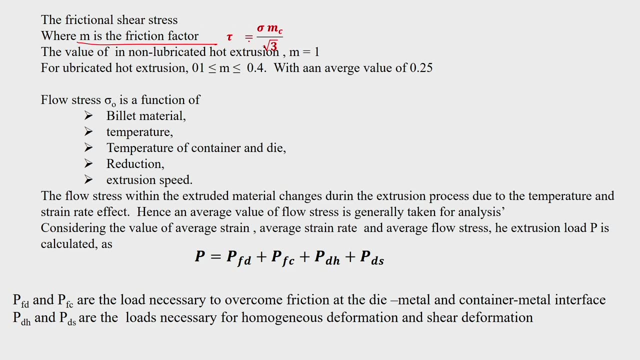 stress, the frictional shear stress toe. let it be at the work piece metal in the interface or let it be at the work piece die interface. So we in most of the case particularly hot working operation when we look at it. we define the toe as that is a frictional shear stress. 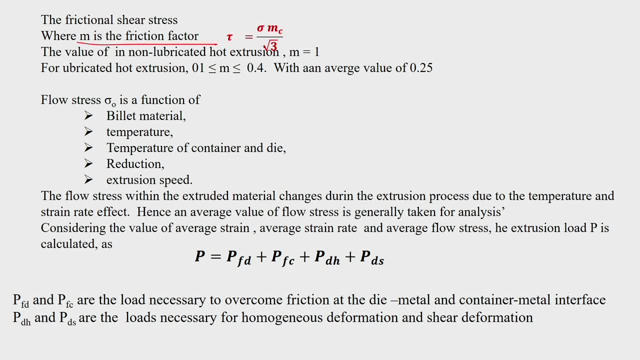 The interface toe near to the interfaces sigma m, c by root 3, so basically it should be sigma 0 uniaxial process into m by root 3. c has no meaning. actually c is whether it is at the container billet or whether it is at the die billet. when it is at the container, 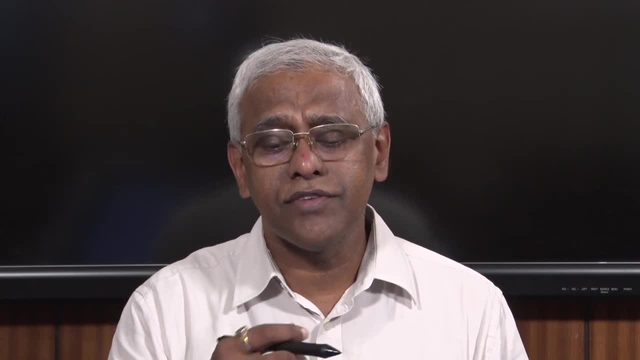 billet, you call it as m c. when it is at the die and the billet interface, you call: just do it as. But in general we can say the- this is the thing- uniaxial process. So it is a frictional shear stress. 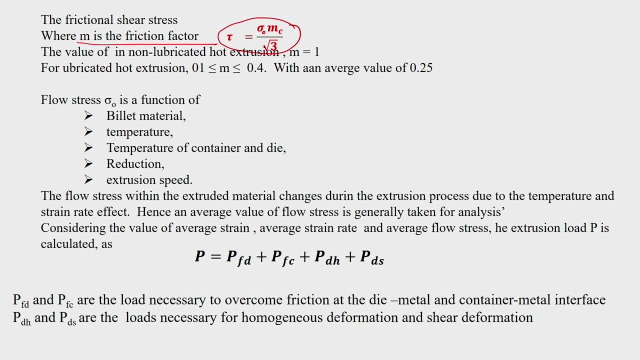 It is a frictional shear stress. So it is a frictional shear stress. So it is a frictional shear stress at that conditions of temperature and strain rate. what is the uniaxial into m by root 3? because the this is mainly the sticking friction which 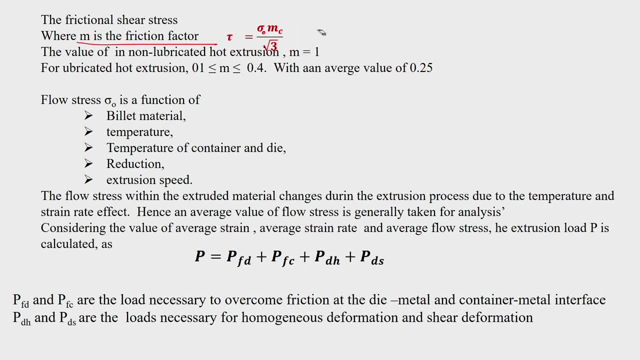 is coming into picture And the value of m, value of m generally. for a non-lubricated hot extrusion process, it is taken as perfect sticking friction, that is, m is considered as 1 and for a lubricated hot extrusion. For lubricated hot extrusion process, m will vary anywhere between the 0.1 to 0.4 m will. 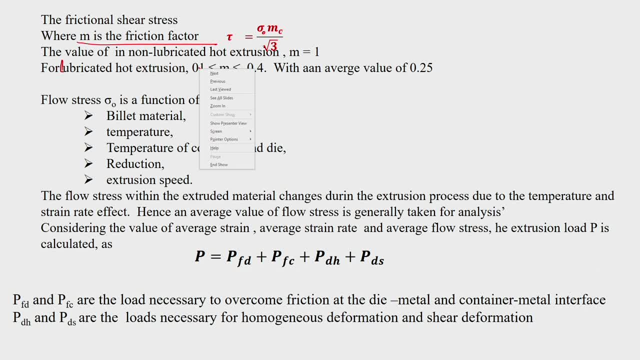 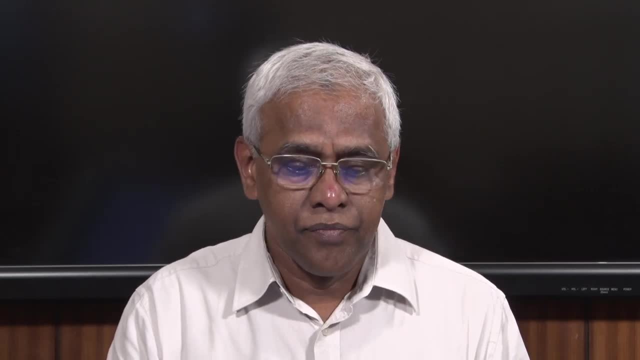 vary between 0.1 to 0.4. okay, And for most of the analysis purpose we can take for a lubricated hot extrusion process, we can just consider it as a value of 0.25. with an average value of 0.25 we can take. 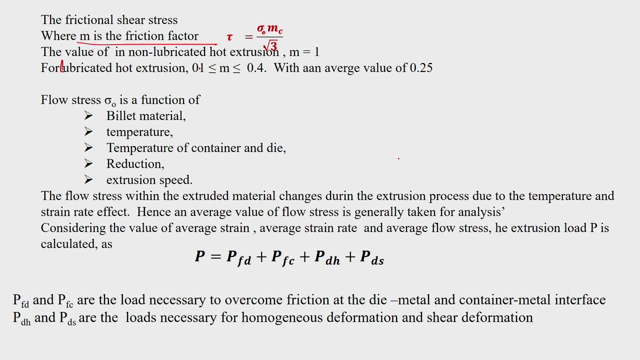 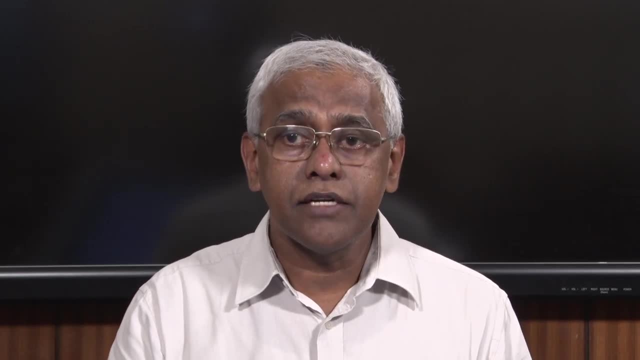 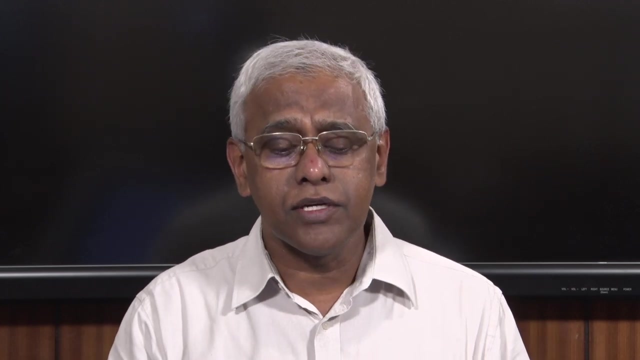 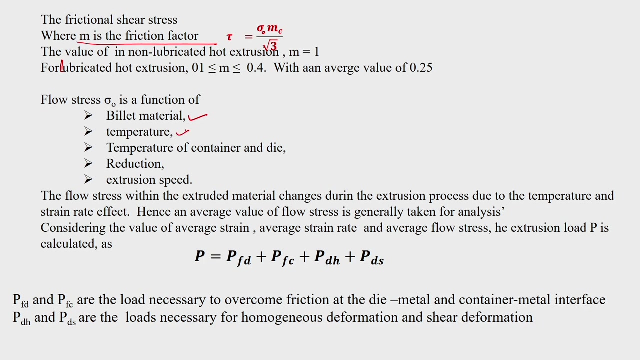 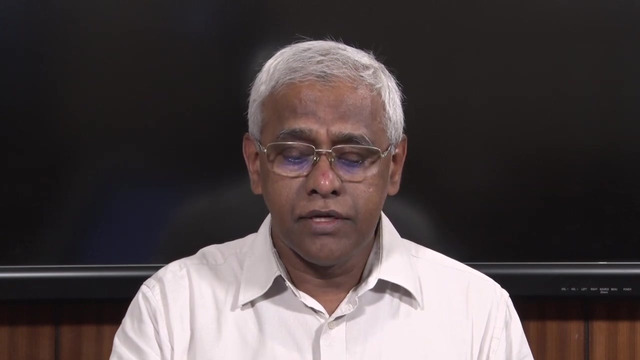 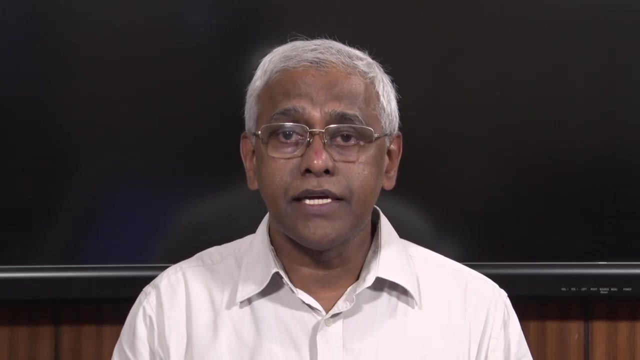 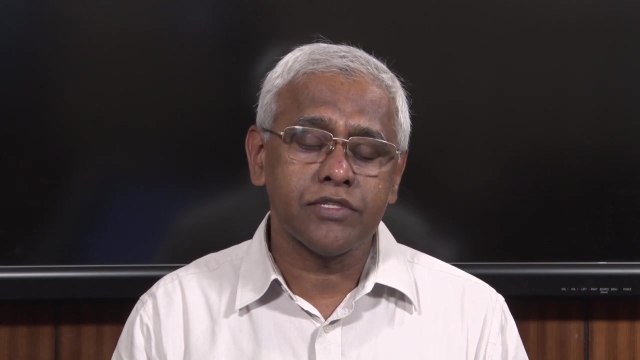 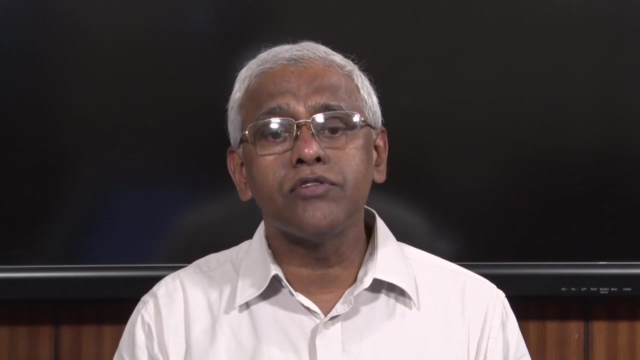 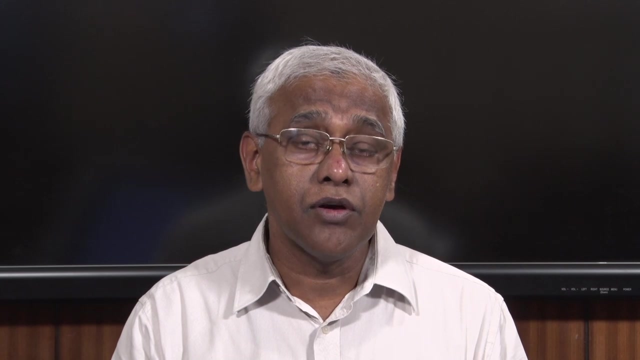 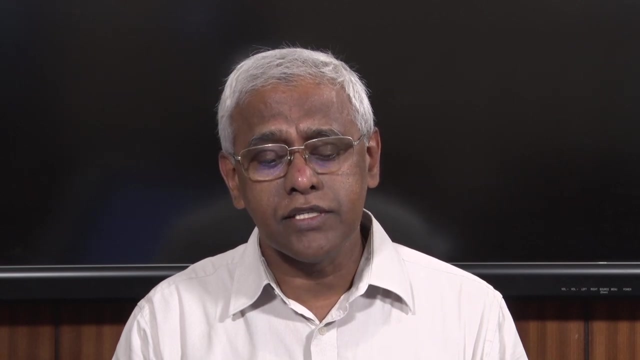 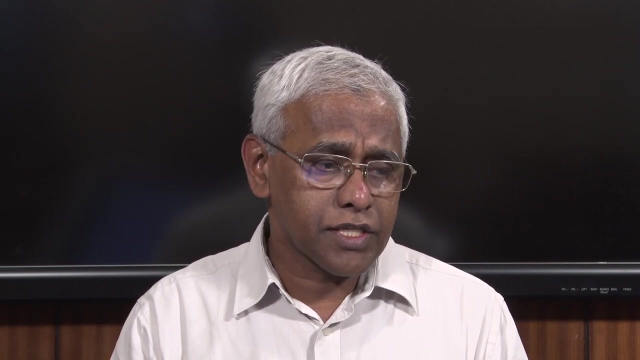 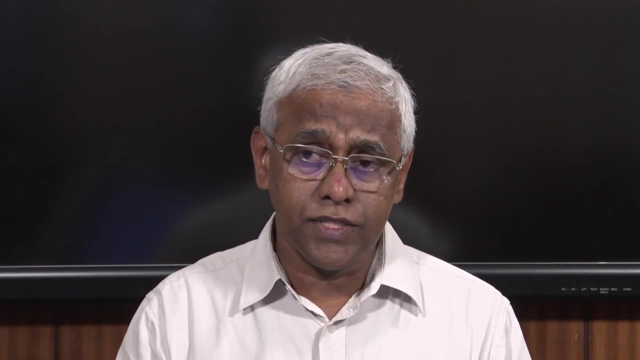 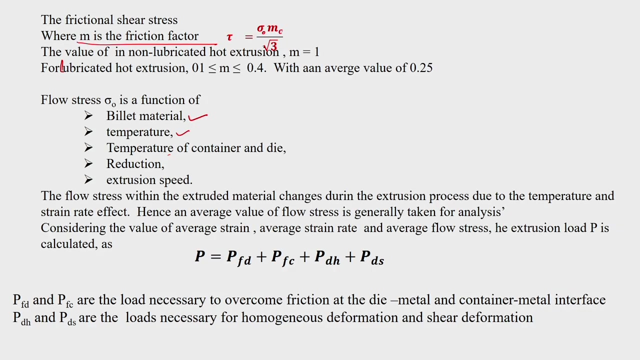 I think it is very important in this cases of extrusion, specially a hot extrusion, Then frost stress also depends upon the reduction. the higher the reduction, the frost stress will be high at the outlet. And another is the extrusion speed, because depending upon the extrusion speed, the metal 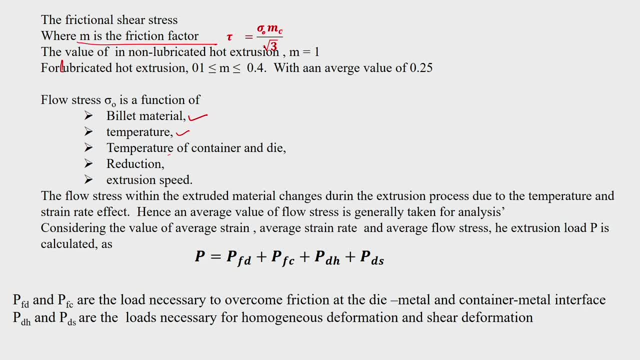 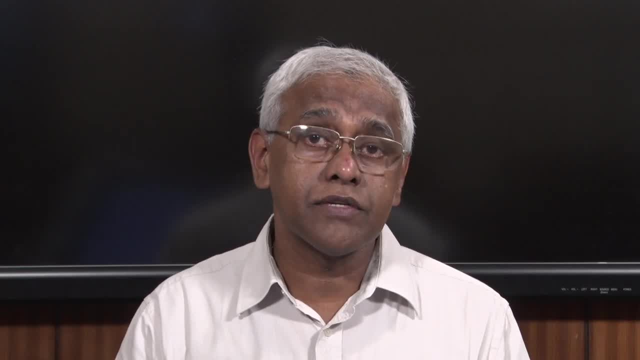 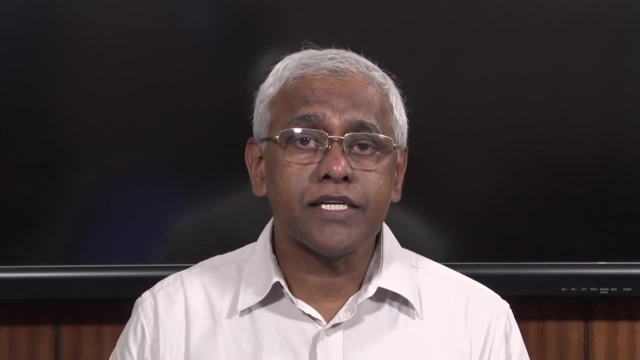 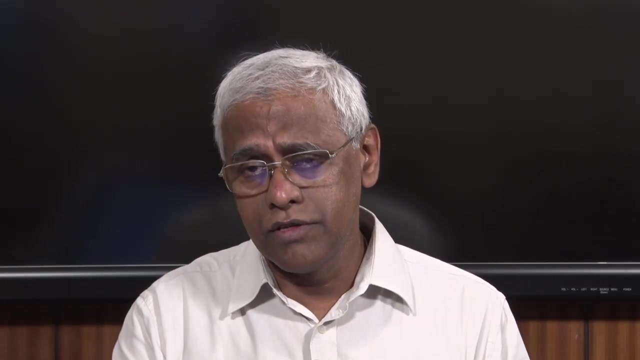 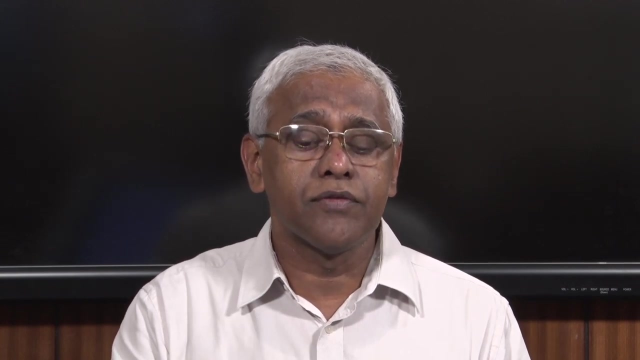 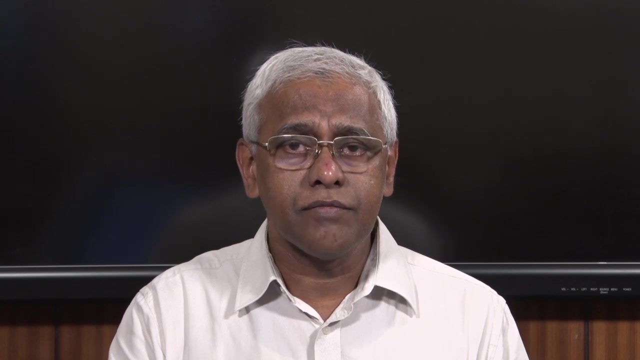 moves through the deformation zone and in that process the strain there keeps on changing and sometimes now you will find that there is an order of difference between the strain rate, BETHUI. The speed also matters. kansomet a high speed. With higher speed there is going to be defect, and with the lower speed that means lower. 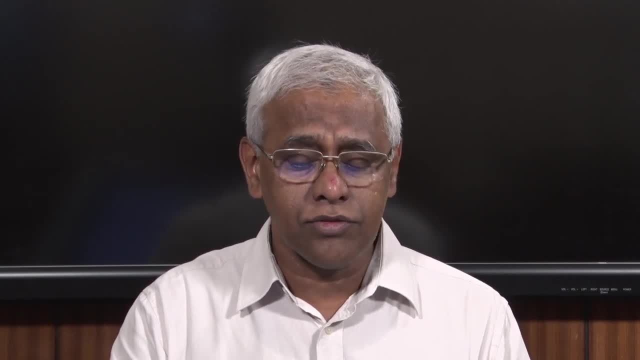 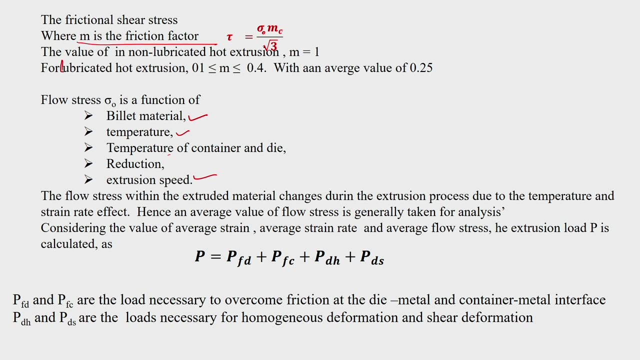 strength rate trees might be. defect may be. yes, so the extrusion speed also has a important influence on the flow stress of the material. Now, the flow stress within the extruded material, the flow stress changes during the extrusion process due to the temperature and the strain rate effect. that is what I was telling inside. 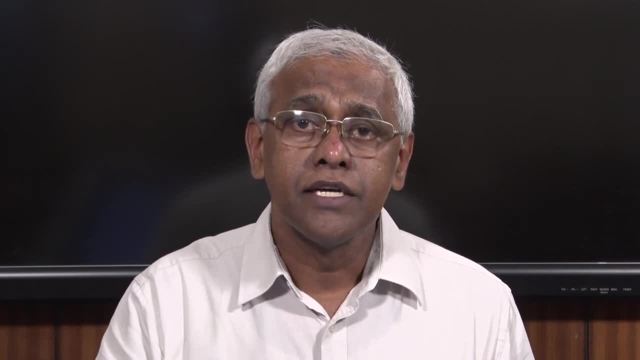 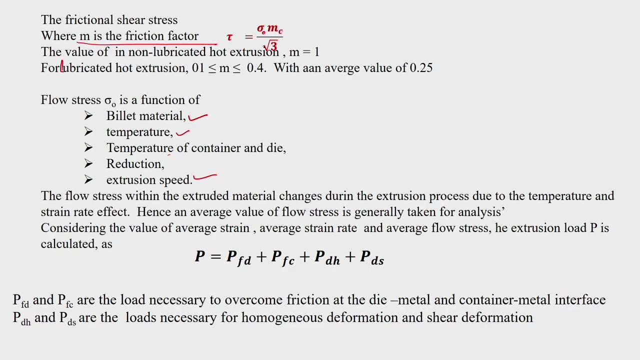 strain rate may be something, but outside strain rate, towards the end of the die the strain rate will be very high. ok, Hence an average value. because these things are changing, so the flow stress based on that may keep varying from inlet to the outlet. So for analysis, 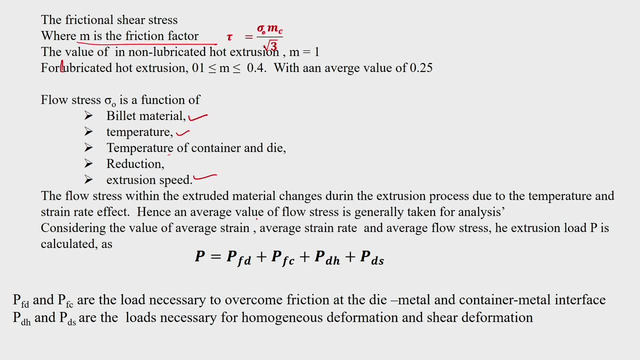 purpose. now we take the average value of the stress that is generally taken for the analysis. ok, and with the reasonable, to a reasonable extent, our analysis with, by taking this average value of strain or strain rate, or effective strain and strain rate, if you take it, you will find that it is very reasonably good ok. 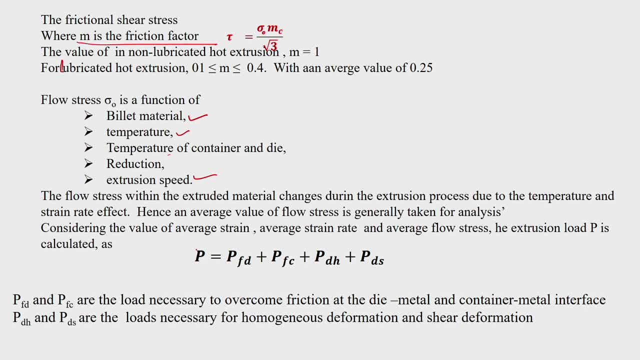 And the extrusion load. when you look at it, the extrusion load P depends upon the load necessary to overcome the friction at the die and the ingot to overcome the friction at the die metal interface. ok, It also depends upon the friction between the container and 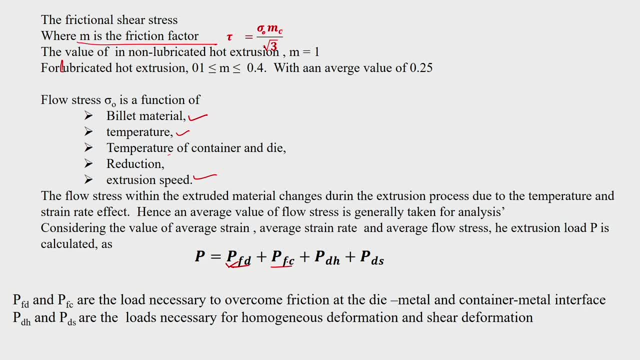 the billet And also the load required for homogenous deformation of the billet inside the deformation zone and also because there is a change in the direction, there is going to be a shear deformation which is taking place. So the total load depends upon these 4 factors and 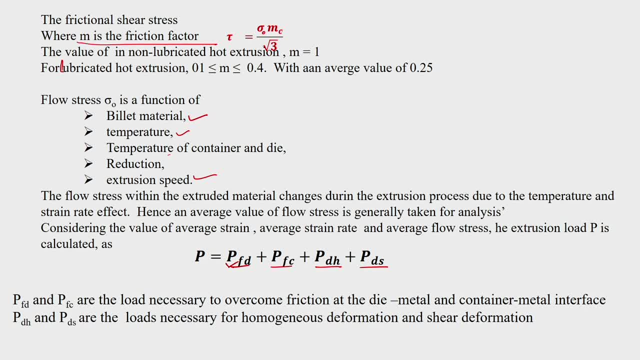 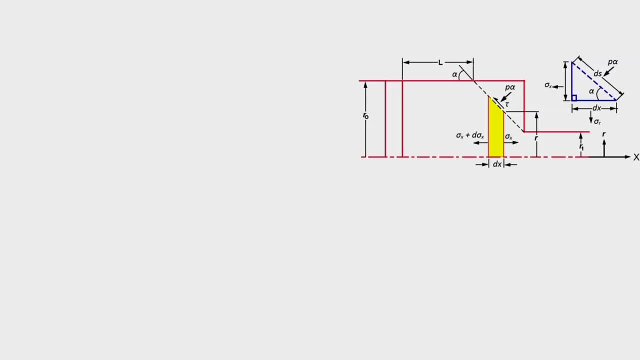 let us now find out for each case how much it is coming. ok, First, let us consider the container friction. So if this is a section of that, you will find that this is your container, this part is your container, which is there. ok, and this is your extrusion die, which is. 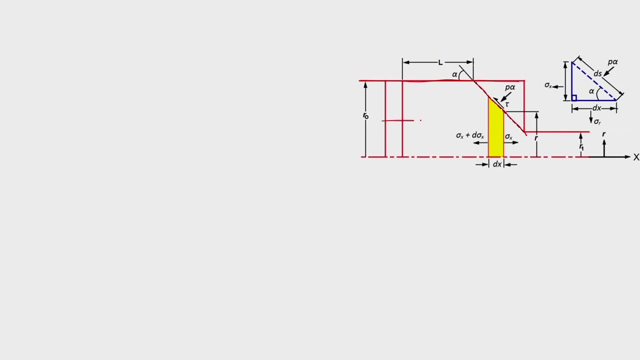 coming here and this is your billet which is going out. ok, when it is moving like this, it moves like this. ok, the billet is. So this is because of the symmetry- isosymmetric case, so axisymmetric case, you know. so we have shown only half of the arrangement, ok, So in this, 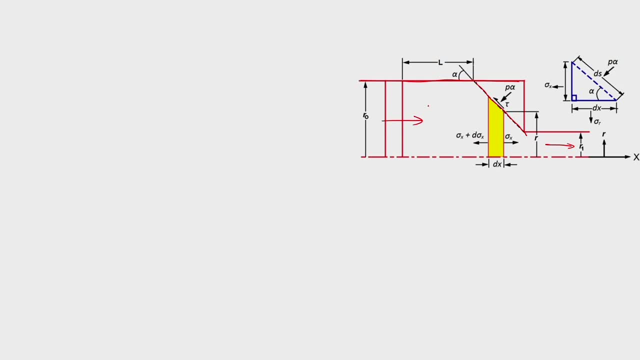 case you will find that the billet is moving like this: ok, So in this case you will find that this is the, this is the billet and this is the container. So the- if you are assuming that the cylindrical portion of the deforming body, because most of the case this container- 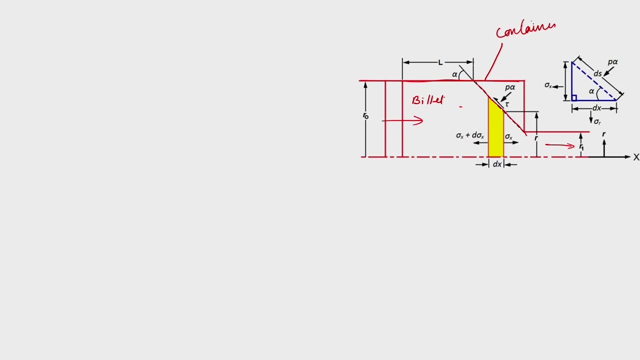 is cylindrical in shape, ok, and the frictional force between the container and the billet- ok- will be experienced. So, at this length, because this is the part which is moving forward from the ram, it is moving in this direction and it is pressing this billet here. So, in this case, what happened? 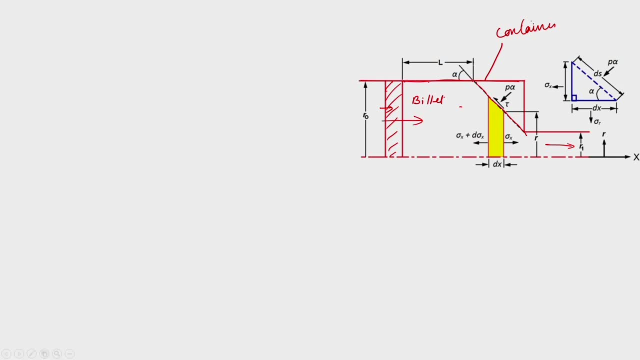 this is the length where the billet is in contact with the container, this overhang length. ok, so over length l, which is given by this l, that is the particular, So the frictional force, the frictional force, so first part, we will just write it as container. 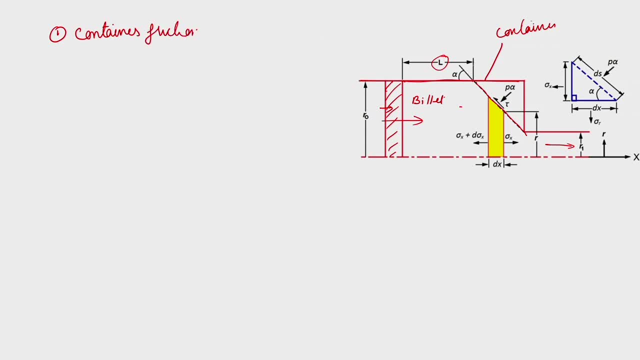 friction, in this the frictional force between the container and billet, Ok, ok, will be experienced at the over length L portion. And so this, the container friction P f c. we can say that this is the line, but since it is a cylindrical in piece, know you can 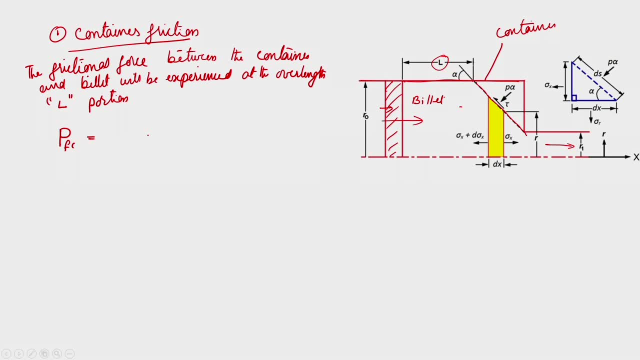 say that P f, c will be the total area which is coming. is pi d into L. what is L? is this one? sorry R 0 is coming here So you can say 2 pi. say R 0 into L, into your tau c where. 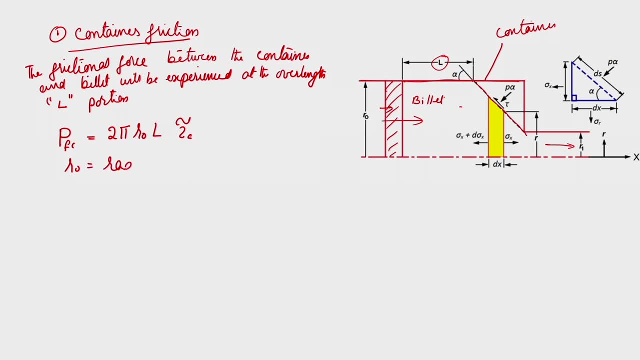 R 0 is the radius of the container And tau c is the frictional shear stress at the container region of billet. And normally you will find that this tau c is equal to, say, m, into which we have discussed okay by root 3.. So this will be your uniaxial flow stress by root 3, where m is equal to: 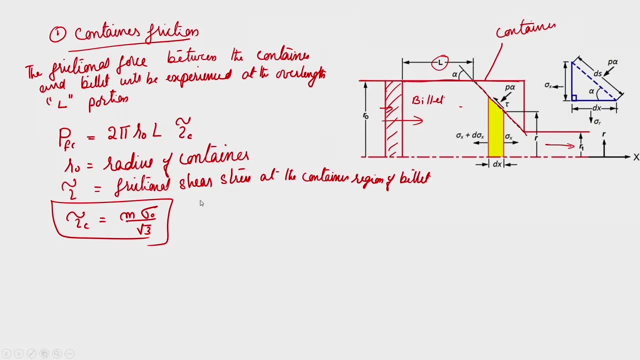 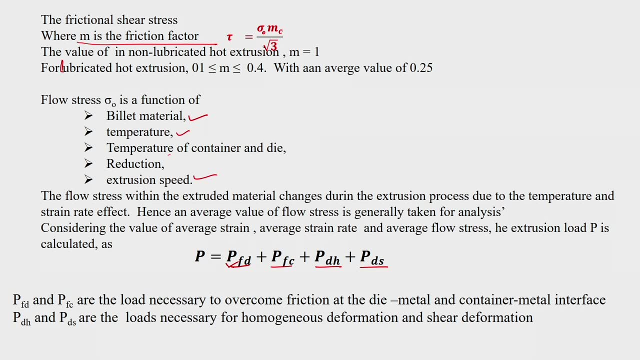 and we discussed that- m for lubricated cases. So for non-lubricated hot extrusion, if it is 1 and for lubricated hot extrusion it will get reduced. m will be 0.1 to 0.4.. So that 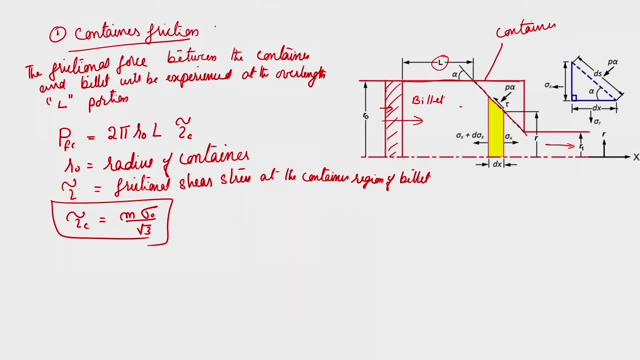 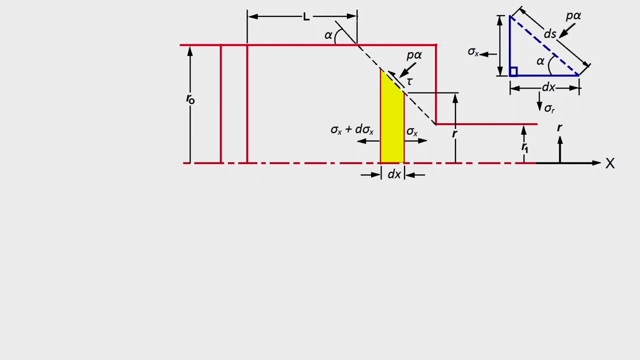 is the thing. So this is how the container friction will take it. So that is the thing. Now, as the forging advances, this total frictional force keeps on reducing because L keeps on reducing. okay, So this will be the initial case, what we have said. Now let us come to. 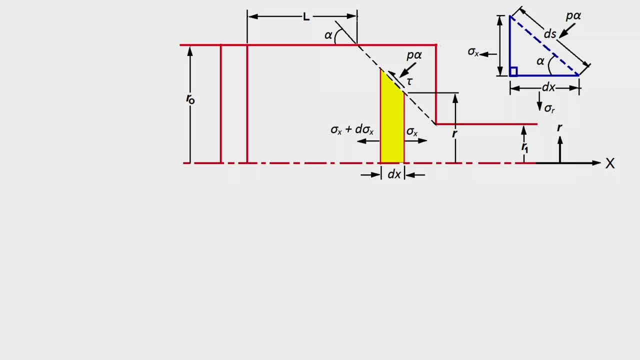 say, force equilibrium in the deformation zone. We have to study at the deformation zone. So the deformation zone is basically a conical section which is shown by this. See, this is your die, So your maybe. this, these from here is your deformation zone, which. 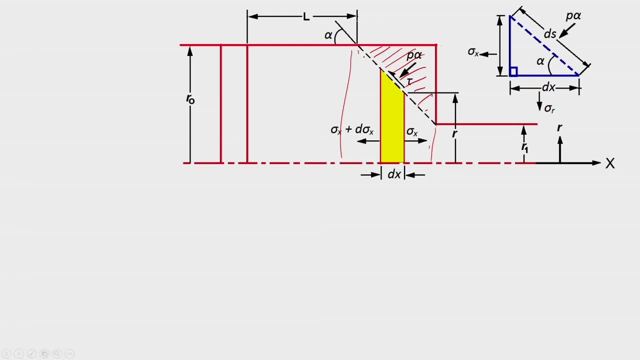 is coming other part. it is not deforming. So this region is the deformation zone. So basically it is the conical section. So we are assuming conical die And so the the deformation zone is a conical section with an intruded angle of 2 alpha. So if you just expand this, this is alpha because 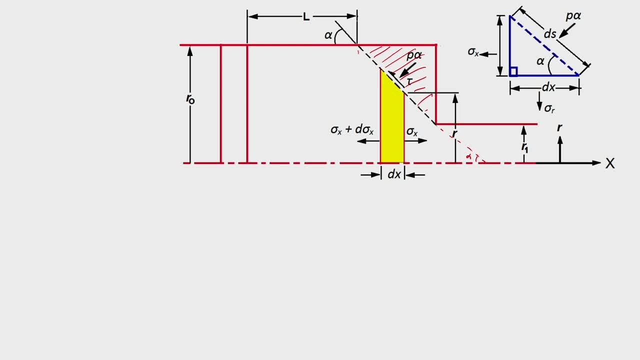 it is symmetric, that will be 2 alpha, So that is 1.2, because it is 0,. right Here it will wonders, here it is just going to scraped. So 2 alpha. So this is called as alpha is called as a semi con angle, semi con angle, that is the thing. 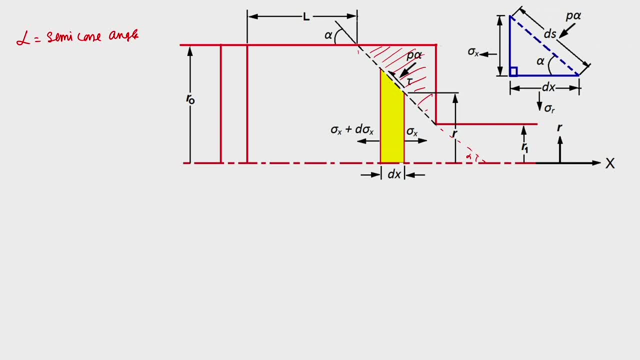 So if you just consider a small strip or a small disc strip or strip at the deformation zone, because deformation zone is from here to here, So from here to here is the deformation zone. So if you just consider a small, infinitesimally small disc of thickness dx, and this is your x. 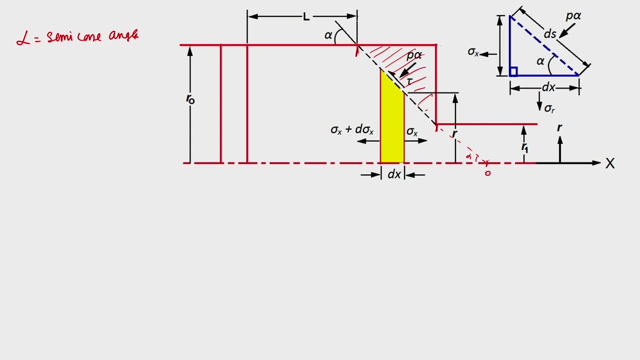 direction if you are telling, and this will be your origin, if you can just consider like that. So this of dx, which is shown by the shaded line, that is, the yellow colored shaded region, is a disc and with the initial part, which is r. here This is the r and you will find. 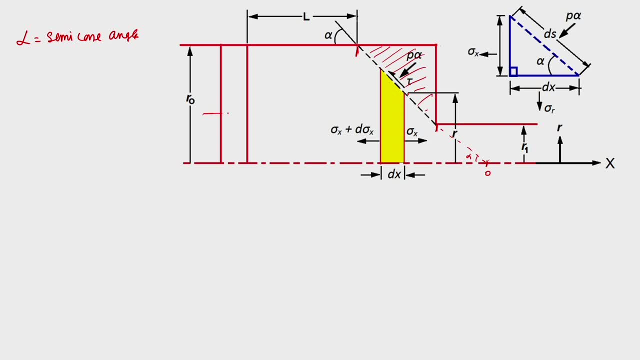 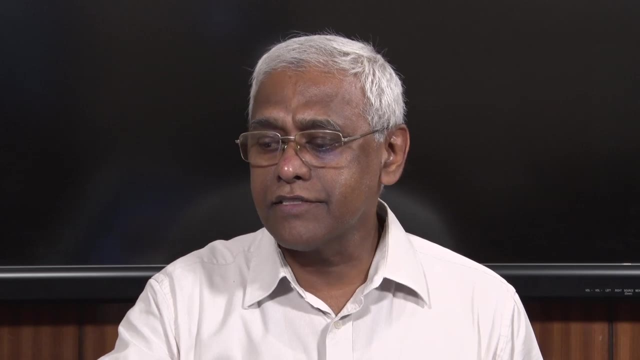 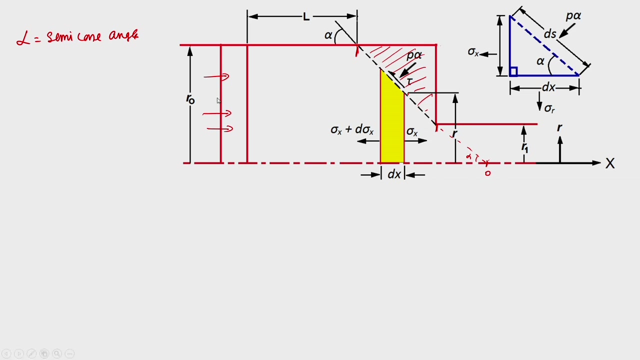 that and you will find that, due to the pressure which is being applied at this region by the ram, There will be a variation in the stress from both the sides of the stress. So let us consider a small strip of thickness, dx along the x direction, along this direction, and then, because of this effect, of this extrusion, 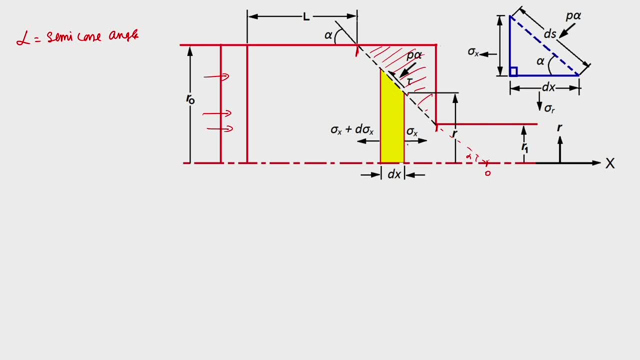 pressure extrusion load. at this, you will find that the stresses. there is an imbalance of that, for if you are considering, there is a variation in the stresses across this small strip and these are the various forces which are acting or stresses which are acting. You will find that there is this p alpha. p alpha is the or the normal pressure acting. 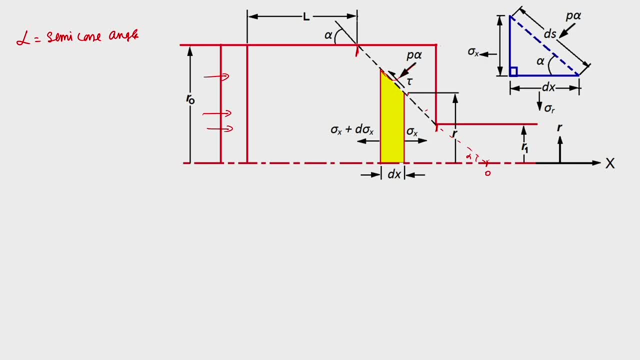 on the interface between the billet and the die and the axial stresses are sigma x plus d, sigma x on the left side And sigma x on the right side and you can see that the various geometric consideration which are there. So axial stress is acting along this x direction and there is a radial 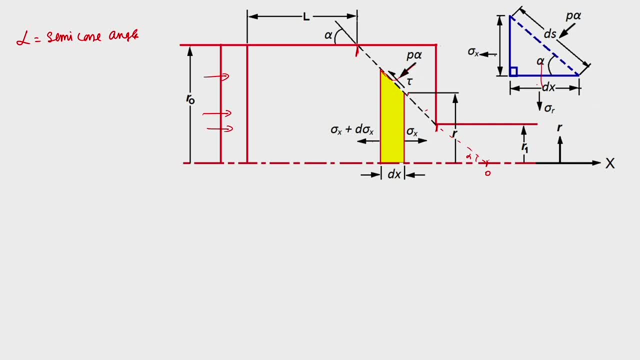 stress acting on this strip also in this direction. So, and various geometrical relationships. we can get it from this Now, if you consider that strip is under equilibrium, under steady state condition, if it is under equilibrium and the equilibrium forces along the x direction. 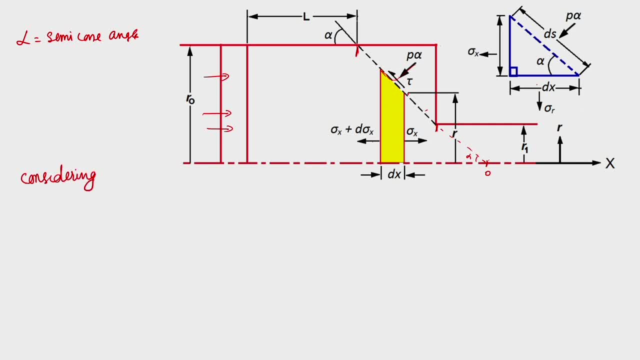 This is possible, but if you consider the equilibrium of forces along x direction, we can write sigma x plus d, sigma x, which is on the left side, integral of sigma x to the lesser side. You can write it along the Die, sigma x that is along the left side, and assuming the general equation for the North. 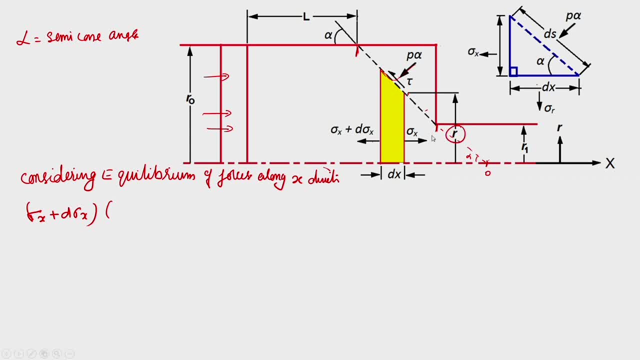 elsewhere along the middle when you now communicate to sigma, this jakby attacked in the associated into the radius is r. this is the radius which is the r plus d r square into pi, the total area it is going to come So minus pi r square on the other side, pi r square, sigma x plus. 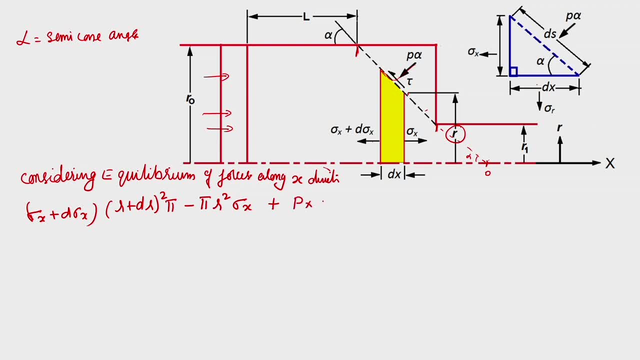 you will see that p into 2 pi r, because there is a normal pressure is effecting its component. you have to take it along the x axis. similarly, there is a shearing stress. shear stress at the interface between the die and the punch, which is represented by toi, is also there. 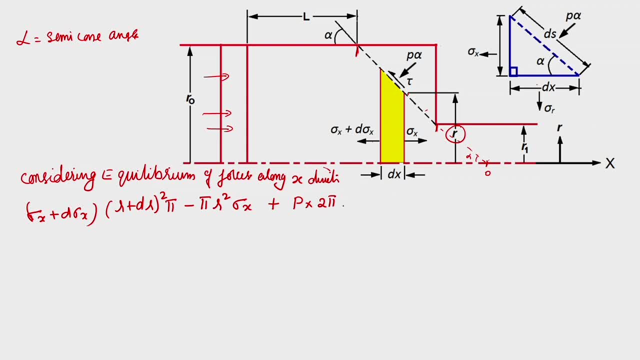 So here, if you look at the normal stress, 2 pi r into d s sin alpha. So you can just look at d s sin alpha is coming here plus tau into the shear stress component if you are taking, taking the component along the x axis, 2 pi r into d s cos alpha. sorry, this is sin alpha. 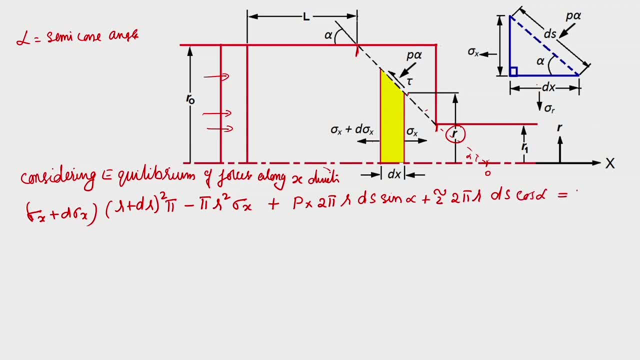 not theta. cos alpha is equal to 0.. We can write equation number 1 where sigma x is the axial stress. I will write: sigma x is the axial stress along x axis and r is the radius of the strip, P is the normal die pressure. 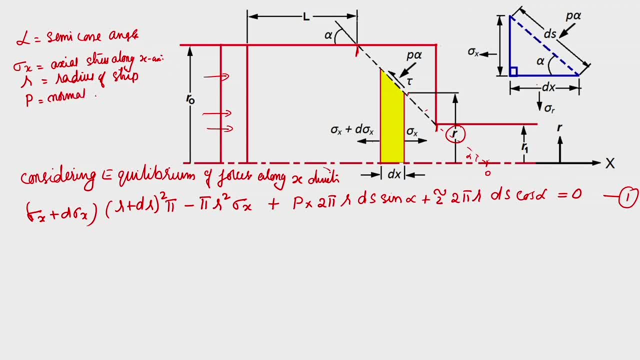 and d? s is equal to the contact length of strip and a die. and from this geometry we can find it as: d? s is equal to d? r by sin alpha is equal to d? r by sin alpha, d by sin d, x by cos alpha. So that way we can write it or we can also tan: alpha is equal to that. 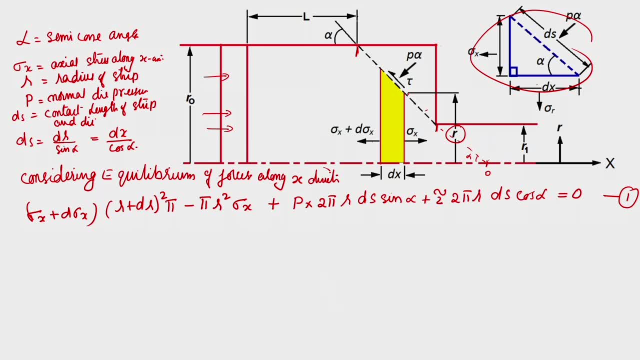 is d r by d x. ok, So that way also we can find it out. So now expanding this equation and neglecting the higher order terms. So expanding and neglecting higher order terms, we can write this, say like: if you expand it now, you will. 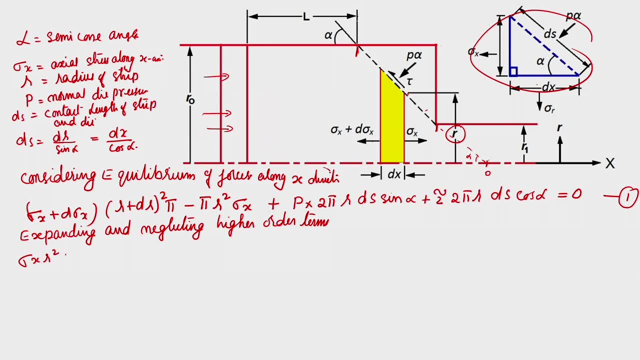 find it as a sigma x. sigma x into r square plus sigma x into 2 r d r plus sigma x into d r square. plus d sigma x into r square. plus d sigma x into 2 r d r plus d sigma x into d r square plus. 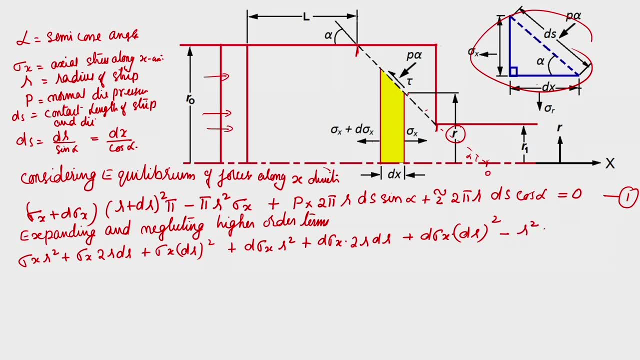 d sigma x into d r square. sigma x into 2 r d r plus sigma x into d r square. plus d sigma x into 2 r d r plus sigma minus r square. sigma x plus 2 p into 2 r d s sin alpha plus 2 r tau into d s cos alpha. 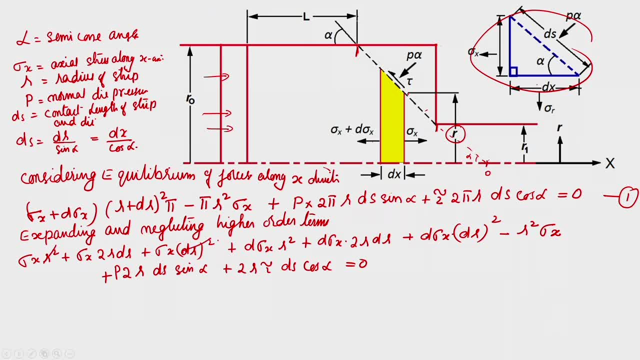 is equal to 0.. So this will go, this will go. this will go. sigma x d r square also will go, because these are the higher order terms and this, also, this and this will go. So this many terms will get removed, So we can finally write it as 2 r, 2 r d r into sigma x plus. 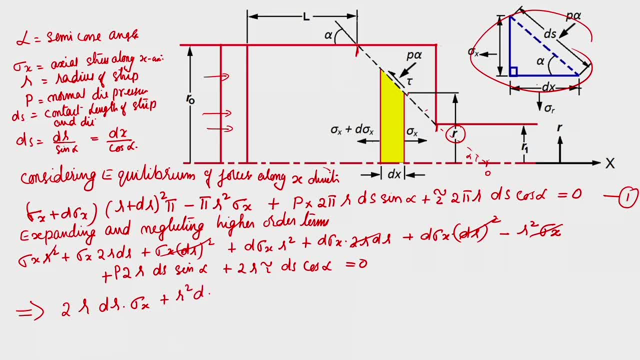 r square d, sigma x. r square d, sigma x plus the last two terms, that is, sigma x plus r 2 p r d s, sin alpha plus 2 tau r d s, cos alpha is equal to 0.. So this is equation number 2.. Now let us consider: this is equation number 2. now let us consider the equilibrium of. 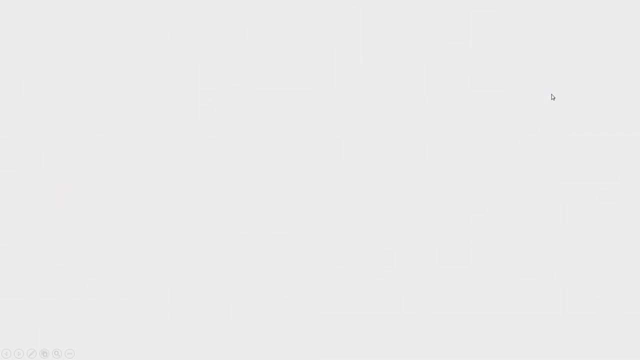 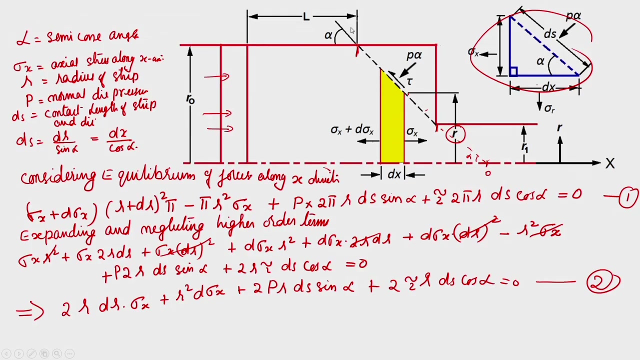 forces in the radial direction, because here also there is a radial direction which is coming, the equilibrium forces of forces in the radial direction, So that if you look at it, there are what are the terms which are coming. So one is the p, ds, cos, alpha. So this, this part, 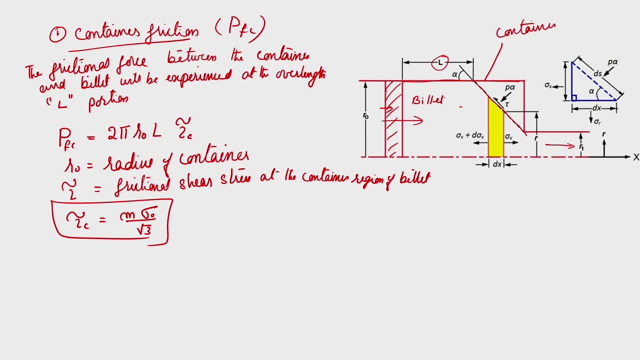 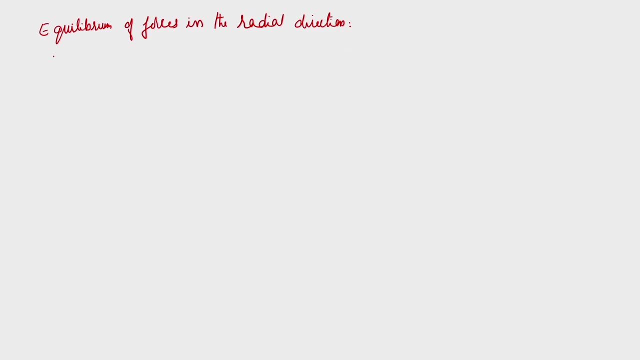 if you resolve it in this direction, that is coming, then sigma r, this sigma r component, also coming, and then you will have this component of this frictional force at the interface, So that these three, if you write it, you can write like that: p, ds, cos, alpha. 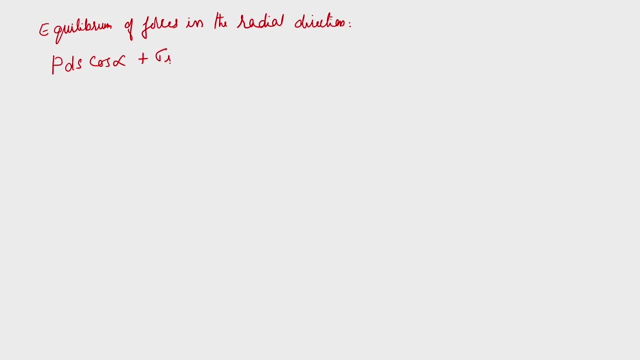 plus sigma r, dx, that is equal to tau, ds sin alpha. So that is because say like: if you write dx is equal to ds cos alpha, that way we can write: since dx is equal to ds cos alpha, we can write that p is equal to. in a simplifying 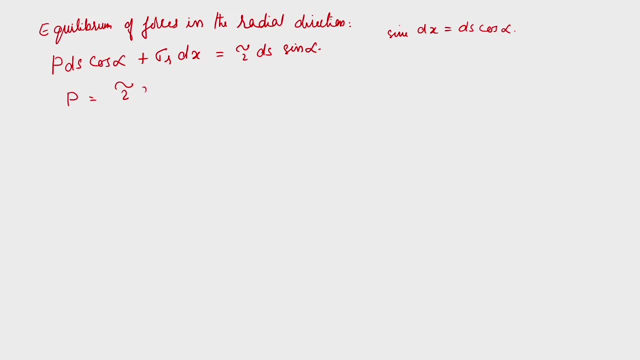 So simple mathematical manipulation. we can write it as tau ds sin alpha by ds cos alpha, plus sigma r into dx by ds cos alpha. So this- and this will get cancelled- is equal to tau tan alpha. Ok, Bell Lettuce. 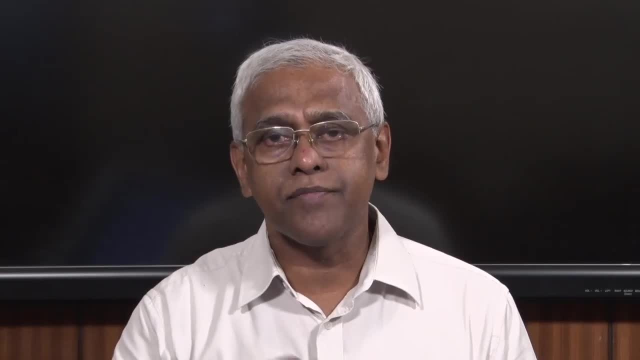 Lecture 9. So if you look at we, we were just considered the considering the case for a cylindrical billet and extruded piece is also cylindrical in shape. This is the simplest, simplestome simplestcase. we were considering it. So in that case, because this is axisymmetric, So 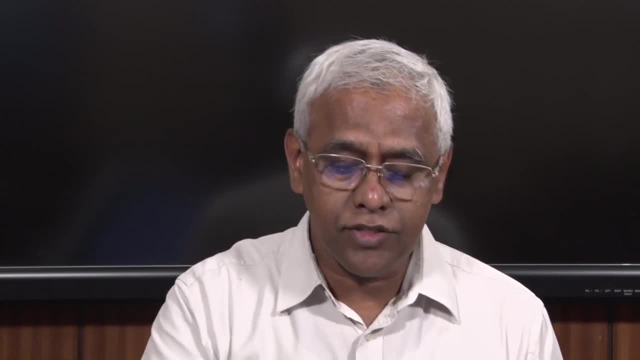 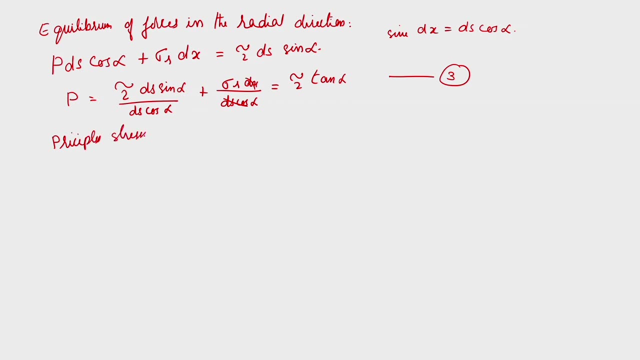 you will find that the principle stresses can be assumed as So: this is that principle stresses we can consume. assume as Bell Lettuce: as sigma 1 is equal to sigma x, sigma 2 is equal to sigma 3, that is equal to sigma r. 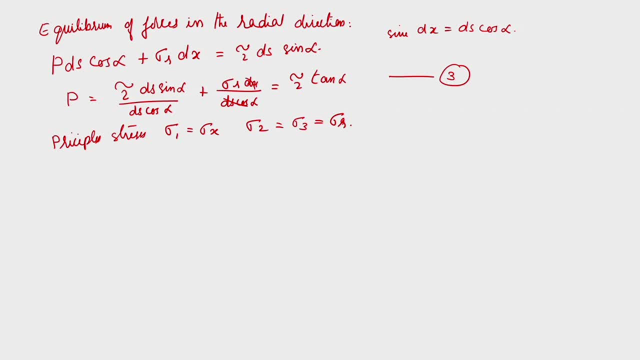 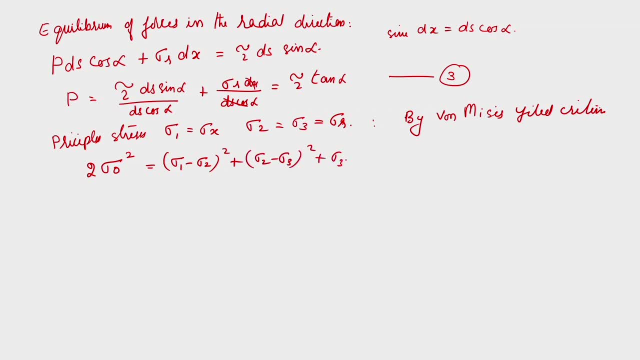 x. sigma 2 is equal to sigma x. sigma 2 is equal to sigma x. sigma r is equal to sigma 3, the whole square, plus sigma 3 minus sigma 1, the whole square, So that if you substitute this value, that is sigma x minus sigma 1, the whole square plus sigma r minus sigma r, the. 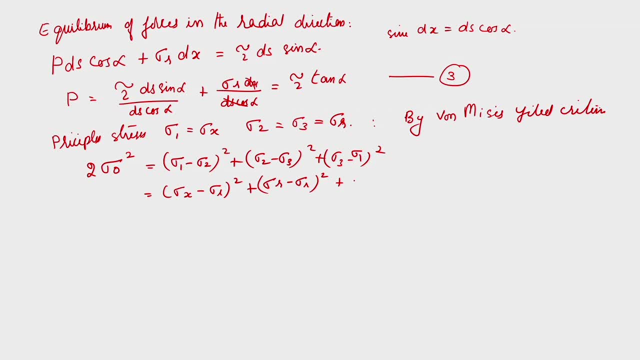 whole square plus sigma r minus sigma x, the whole square. So that will lead you to sigma 0. square is equal to sigma x minus sigma r, the whole square or sigma 0. that uniaxial yield strength of the material is equal to sigma x minus sigma r. So this relationship 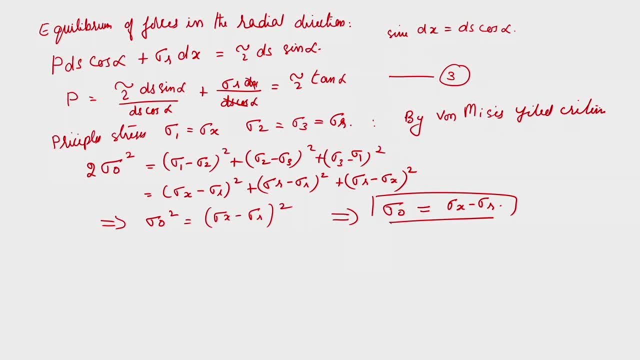 we are getting as per the one misses criteria. So from that, if you substitute into equation 3. So equation 3.. So equation 3.. So equation 3, if you substitute that, we will get it. as p is equal to tau tan alpha say. 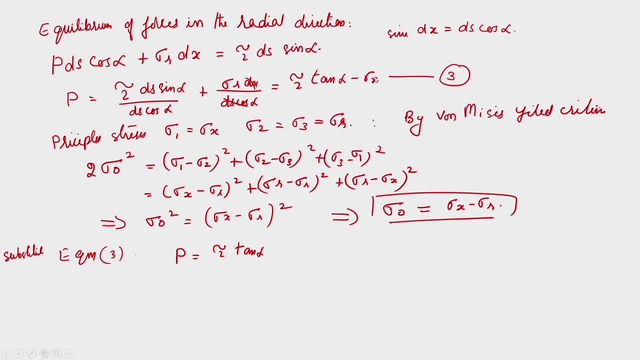 minus sigma r. tau tan alpha minus sigma r is equal to sigma x minus sigma r. So this is the relationship we are getting. or that is: p is equal to tau tan alpha plus sigma 0 minus sigma x. this we are getting. So this is the relationship we are getting, or that is p is equal to tau tan alpha plus. 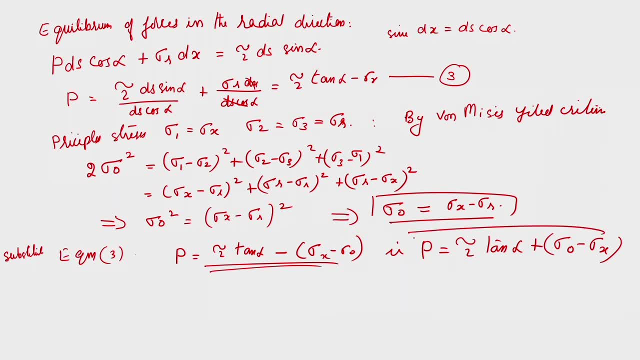 sigma 0 minus sigma x, This we are getting. ok, P is equal to tau. I will write it as equation number 4. that is, p is equal to tau, tan alpha plus sigma 0 minus sigma x. So this is equation number 4.. Now substituting equation 4 into equation: 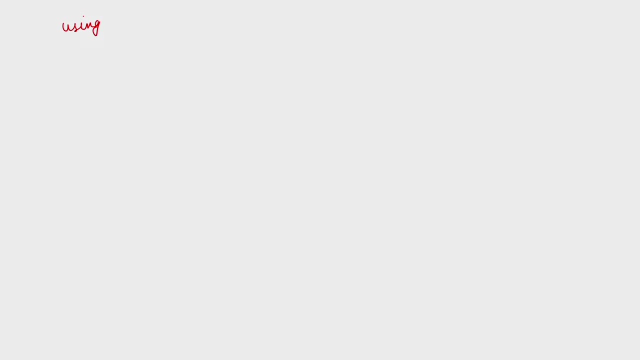 3. using equation 3 and 4, we will get results in: 2 r d r- sigma x plus r square d sigma x, plus r square d sigma x. d sigma x. 2 p r d r, 2 p into r d r, plus 2 r into tau into d r by tan alpha. This is basically d. 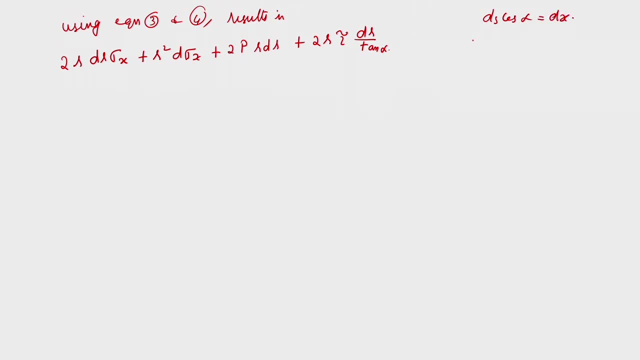 s cos alpha is equal to d x and d x is equal to d r by tan alpha. So when you substitute this, we can- we will get this term from that geometric relationship itself, which I have written earlier. So just to remember here I am just writing it. So that means this: 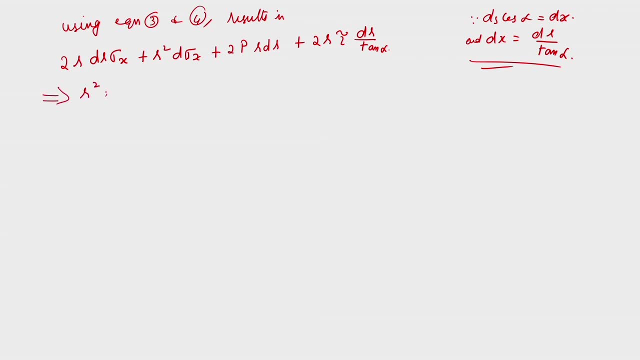 relationship. from that we will get it as r? R square d sigma x plus 2 into tau, tan alpha plus sigma 0 r d r plus 2 r d r into tau by tan alpha is equal to 0. And just rearranging so that means we are getting d sigma X r r is common and everything. 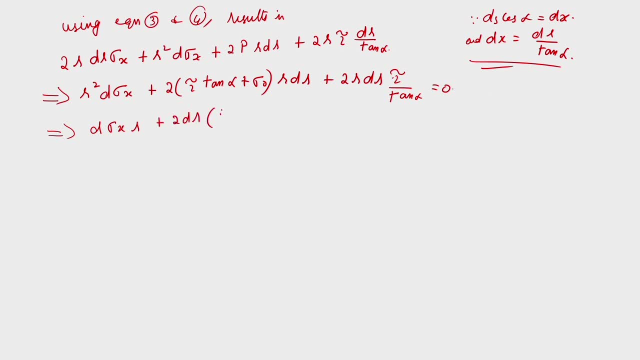 if you cancel, it is equal to tau d r into tau tan alpha minus sigma 0 plus tau by tan alpha is equal to 0.. So that means in the differential form we can write it as d much per by tau r into tau r x, this successful metric 국 to r into tau. 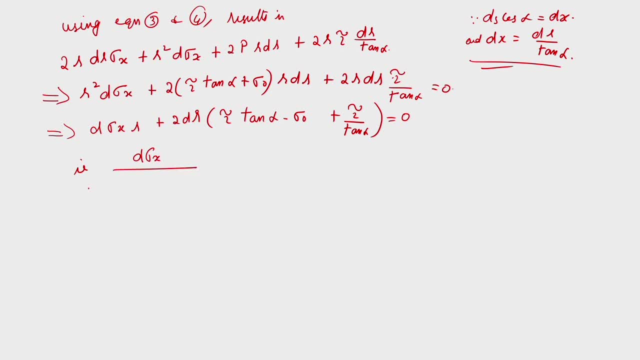 r minusикma x 0 plus tau by tan alpha, which is equal to 0.. And Choice S we will write: is sigma x by 2 into tau tan alpha minus this term we are bringing at the denominator. sigma 0 plus tau by tan alpha is equal to minus d r by r. this is the differential equation. 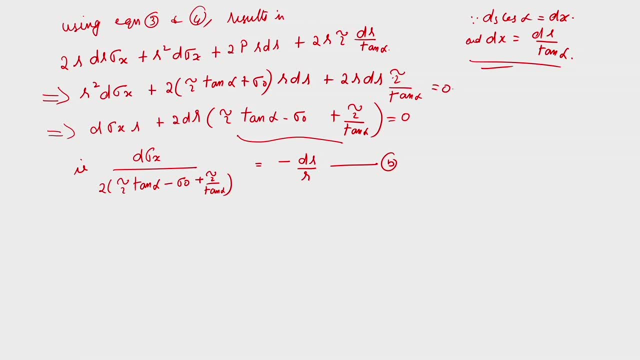 you solve for this and we can get the value That means if you integrate it, integrating equation 1 in equation 5.. So you will get it as: sigma x By tau tau tan alpha minus sigma 0 plus tau by tan alpha is equal to minus log r plus. 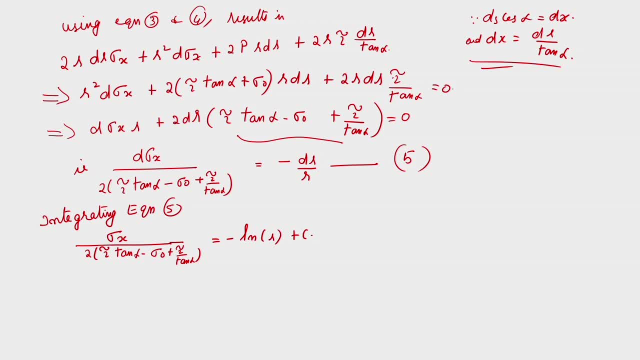 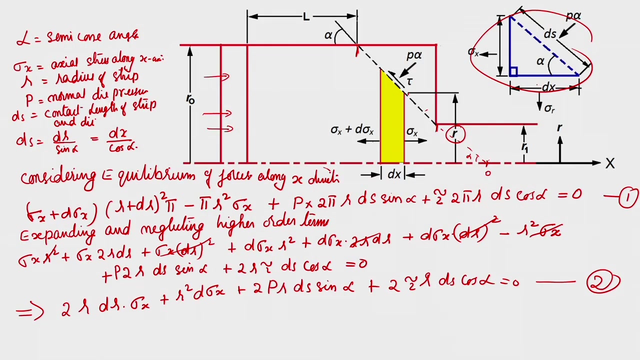 c or sigma x is equal to 2 into tau tan alpha minus sigma 0 plus tau by tan alpha into log r. if you put this as minus sigma x, So this is equal to the exit side. So at the exit, when you are applying the axial stresses, 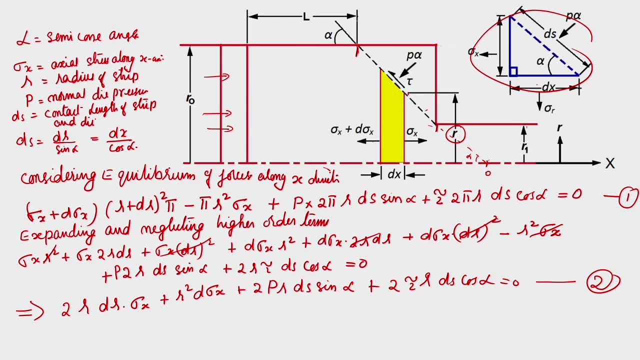 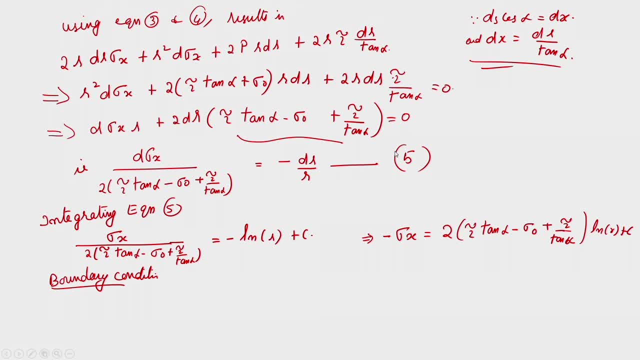 are 0. only inside the die, only the stresses will come. but once it comes out of the die the axial stresses are 0. So that is one boundary condition. So that means at a, at the, at the entrance to the die, at 1, at r is equal to r1, r 1, that is sorry- at die exit. 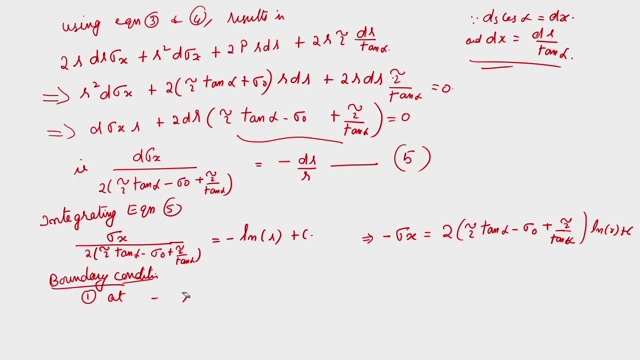 r is equal to r 1 and sigma x is equal to 0. So this, you write it as equation 7 and this is equation 6.. So equation 7: if you substitute from that, you will find that c is equal to. so this is: 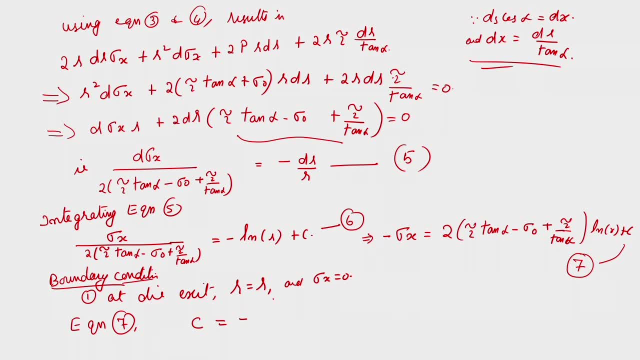 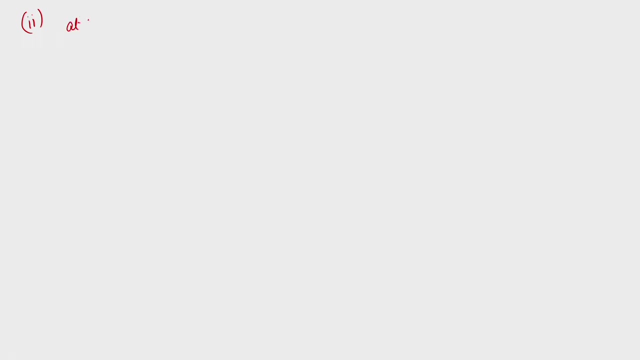 0.. So c is equal to minus 2 into tau, tan alpha plus minus sigma 0.. So sigma 0 plus tau by tan alpha log r 1.. So this value and you apply the second condition, that is, the second boundary condition, is that at the entrance to the die, at the die entrance, 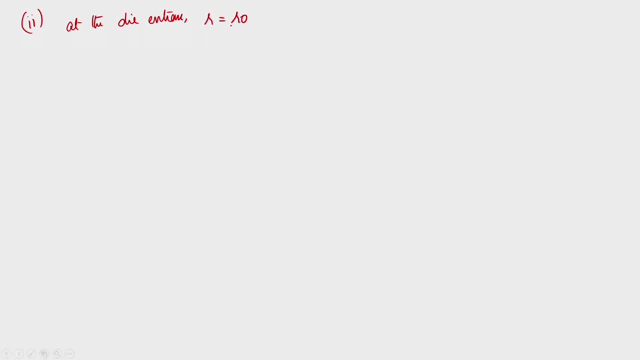 r is equal to r 0. that is the billet diameter, billet radius. So radius is equal to billet radius and the extrusion load, because that is the load which you have to apply, or extrusion pressure when you wanted to. extrusion pressure we have to apply. sigma x. 0 is equal to, if you substitute the. 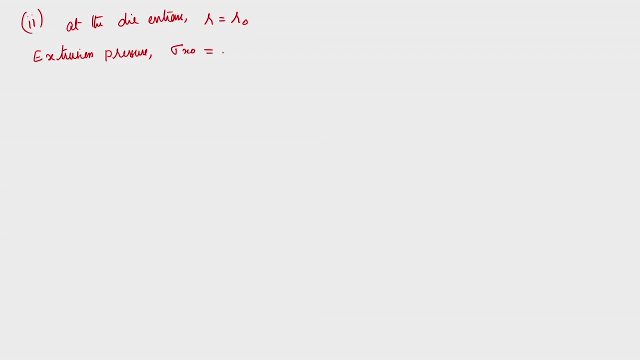 boundary of this one in equation number 6 you will get: that is equal to minus 2 into tau tan alpha plus sigma 0 plus tau by tan alpha. log r 1 plus 2 into tau tan alpha plus sigma 0 plus tau by tan alpha. 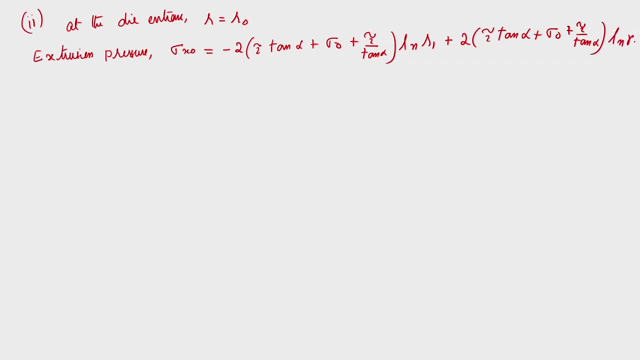 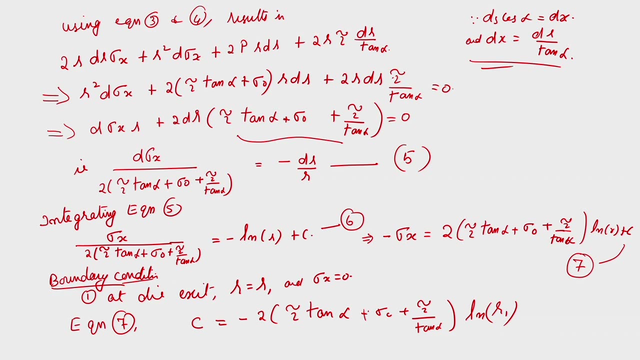 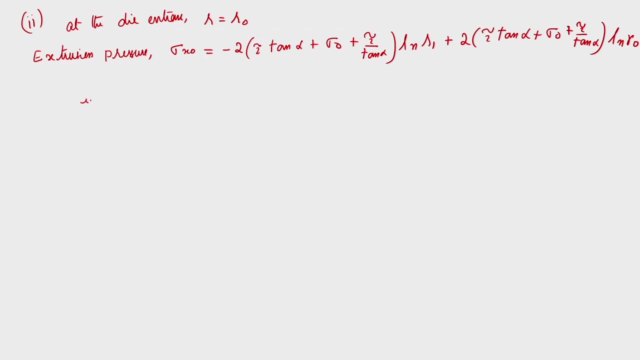 Into log r: 0. here this should be 0 plus. that was a mistake. or that is sigma x: 0, which is the extrusion pressure which you required. we can write it as 2 into tau tan alpha, because just doing a simple manipulation, mathematical manipulation, rearrangement, you will get it. 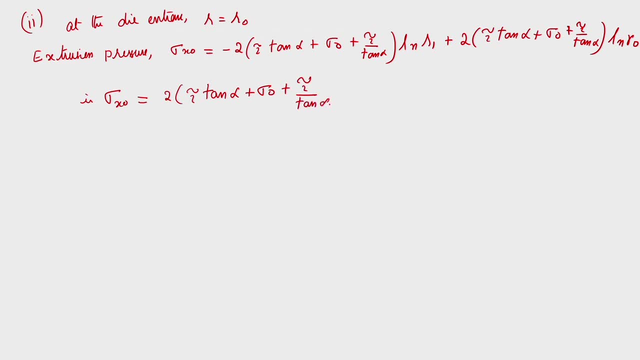 as by tau tan alpha. tau by tan alpha into log r 0 by r 1 or so that is also equal to 2 in terms of area, wise tan alpha plus sigma 0 plus tau by tan alpha, So 2 log r 0 by r. 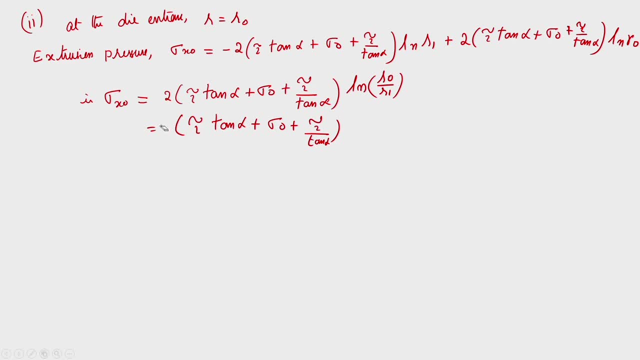 1. So 2 log r 0 by r 1 is equal to log a 0 by a 1, because a is equal to pi by 4 d square. from that you can, since we can write. So that means log 2 log r 0 by r 1 is equal to. 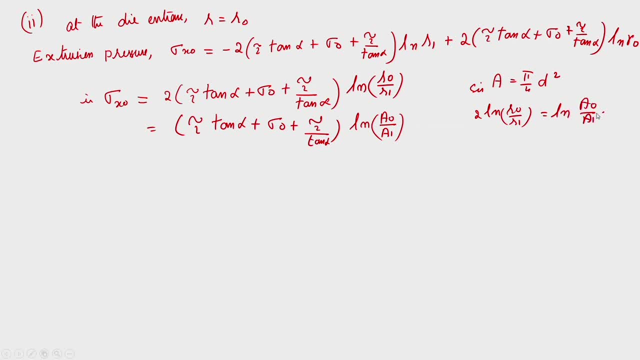 log a 0 by a 1.. So this is your equation number 8, the relationship which you are getting Now. this equation number 8 can also be written in this form: minus sigma x 0 is equal to sigma 0 log a. 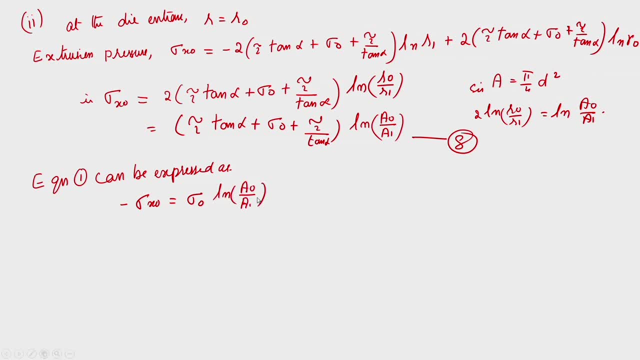 a 0 by a 1. if you just split it and write a 0 by a 1 plus tau, log a 0 by a 1 by sin alpha, cos, alpha. See, in this way we can write it. so which is so? from this, the first part. 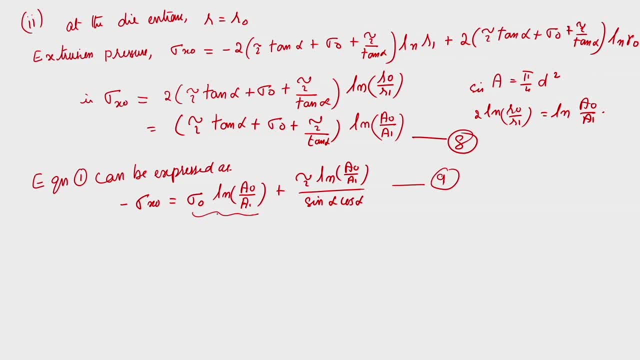 of this equation. this is a stress for homogenous deformation, if I just write it as a, and this is b. So a is the component of stress for homogenous deformation and the b is the component for die of friction at die metal interface. So we can say that: 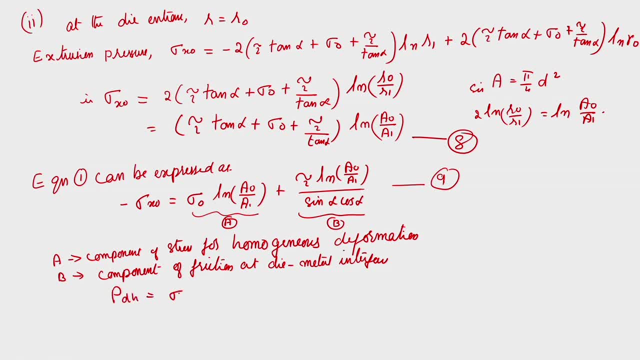 p, d, h, 0 is equal to sigma naught. we can just use it as an average value also because it will vary from inside to outside. So we can write sigma naught log in the generalized way: a 0 by a 1. this is the strain which is there. So effective stress into effective strain. you can say and: 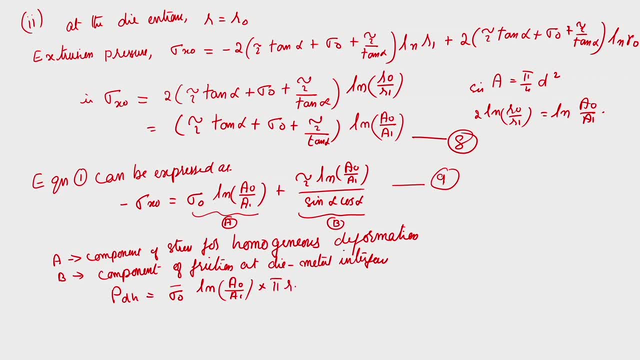 into the cross sectional area, that is pi r square, r 0 square. So this is your equation, number 10 and p f d. So this is the frictional force is tau at the die area. log a 0 by a 1. 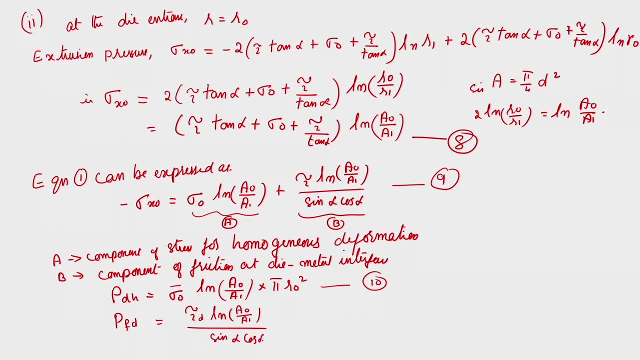 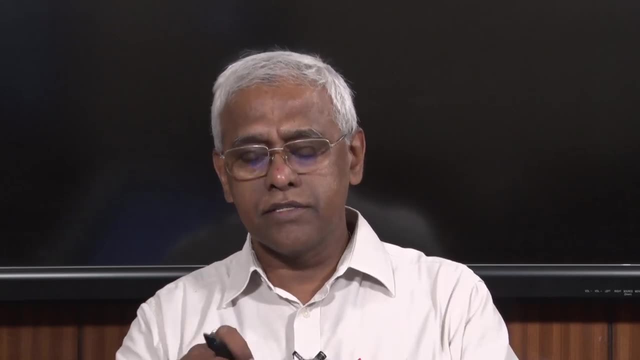 by sin alpha, cos alpha into pi r square, So r 0 square, that is 11.. So these two components we got. third component also we got. So only component which is left is the shearing stress. it is the shear stress which we wanted. 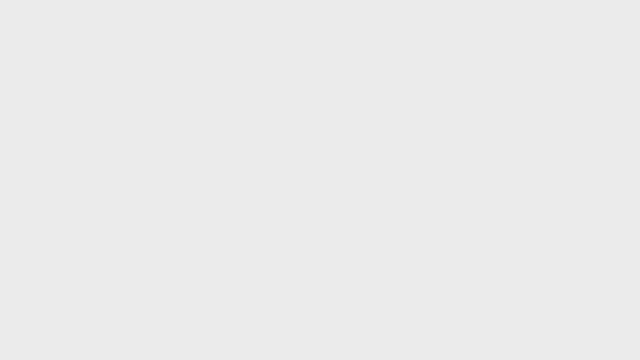 to draw So the stress necessary for shear deformation in the stress for shear deformation in your deformation zone. So if you just take this as the alpha value, let me extend it somewhere here So that it comes this we can assume as the origin. 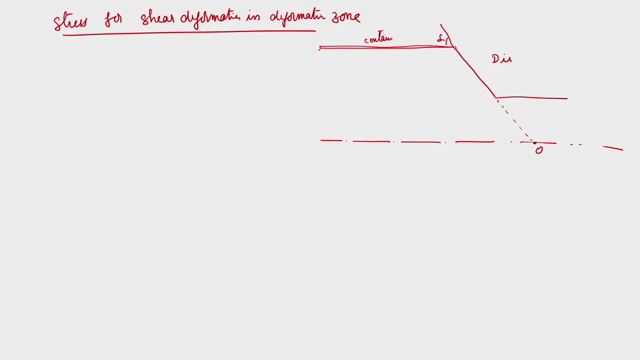 of this. So here it is r 0, that is the billet radius container diameter. also we can say: and this is your r at the exit, r 1 at the exit, So this distance, So this is the die. r 1 at the exit, So this distance, So this is the die. So this distance, So this is. 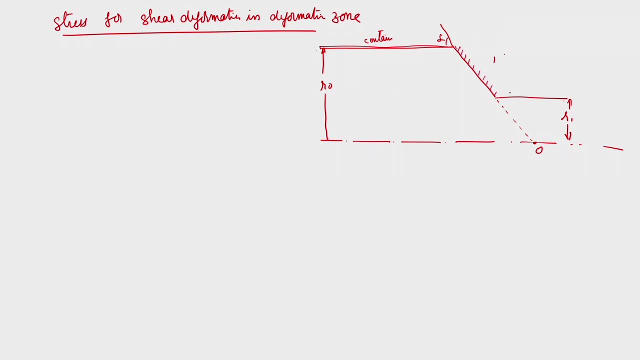 the die, let us say, may be this length. if it is r, This is your alpha. and when the metal is flowing in this direction, when it comes here somewhere, it will change its direction of flow, and it will you. we assume that it is flowing parallel to the die surface. die interface. die work piece interface. 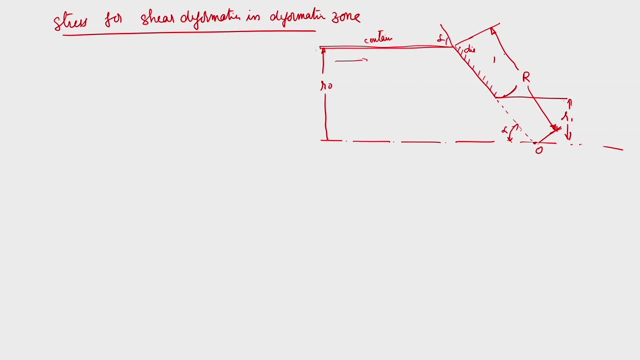 So we can say: there are the material undergoes non homogeneous shear deformation, and shearing is taking place with the center as O and we can just assume, for our simplicity, this is the area. the moment it crosses this region, there is going to be a change in the direction. 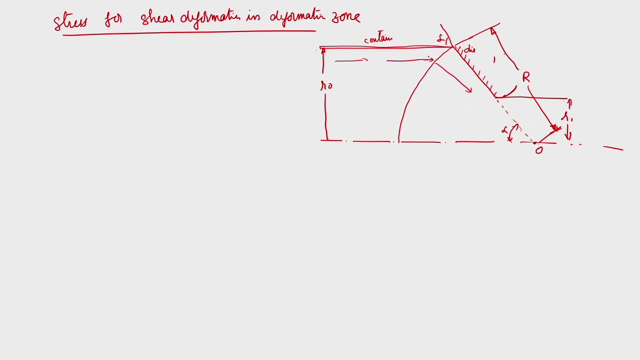 So if it comes like this, and then you will see that change in the direction, if it comes here, there is a change in the direction. if it comes here, there is a change in the direction. So this is how the so there is a going to be a velocity discontinuity when you cross. 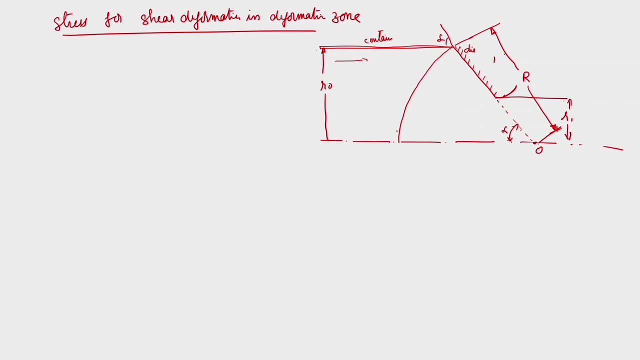 this region and the discontinuity surface. This is the discontinuity, So this is the discontinuity surface which is there, which is shown by this. So across this surface there is going to be a non homogeneous shear deformation and the energy and the load necessary for this we have to estimate. and similarly, when it 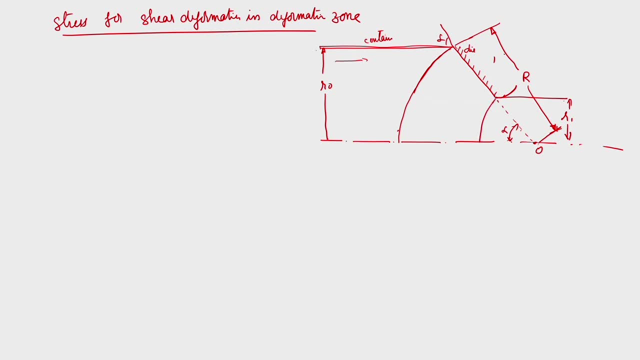 comes to exit, then here also we are assuming there is another velocity. discontinuity is coming here because after this it is assumed that there is no metal flow is in the initial direction. So so our horizontal velocity is coming here. velocity of metal flow when it is moving here it is your v 0. So let us take an arbitrary. 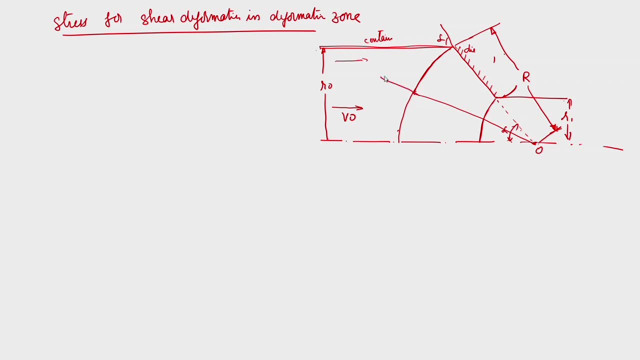 point which is there. So where the radius is r, to get the relationship where the radius is r and normal to this at the, you take this component. one is normal to the surface and another is parallel to the surface. So this is your v 0.. So this is v sin alpha, v 0 sin. 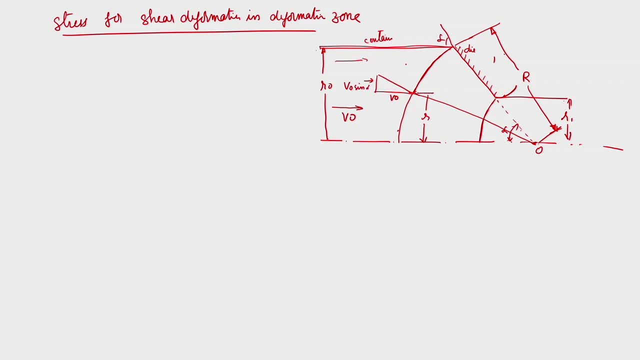 alpha and this is v 0 cos alpha. So this will be the diagram which is coming. one velocity discontinuity is taking place at this discontinuity surface and say I will just at this surface and this surface. two discontinuity: So there is a as the metal enters the deformation zone. 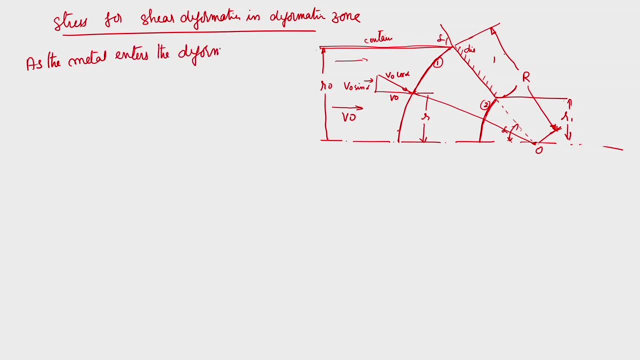 So A tender goes non homogeneous shear deformation And the shear deformation goes w. I can call this, as the deformation, shape and information did not momentum, Okay, Well at the sending occurs suddenly at the assumed discontinuity surfaces say 1 and 2.. So at the entrance boundary, that is at a, at the 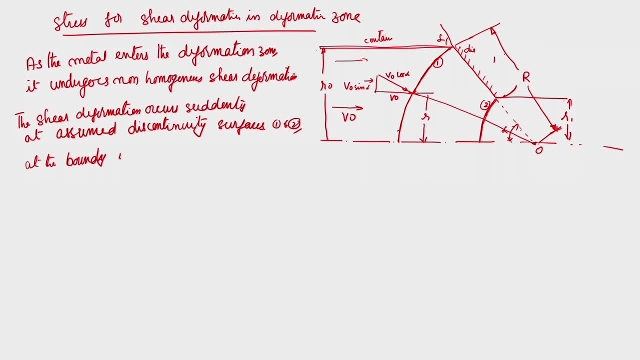 boundary 1. the velocity component normal to a surface is continuous. the velocity component normal to a surface is continuous. the velocity component normal to a surface is continuous. That means it is. this is straight, it is continuous. there is no problem. but whereas if you look, 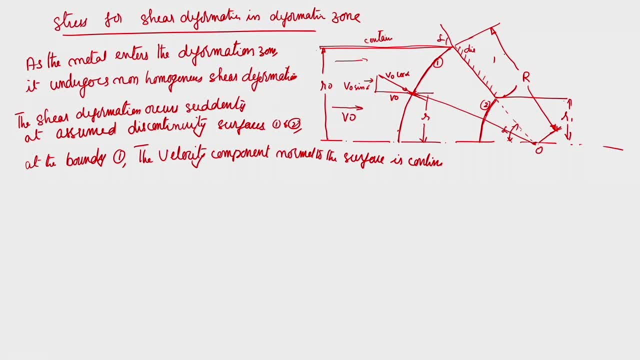 at the velocity, discontinuity at the boundary, which is parallel to that, So that you will find that it is not continuous. So this: there is a small mistake in the way I have written, drawn. it will be fine Here. this is that it is like this: 90 degree is here. So the component at the, the velocity. 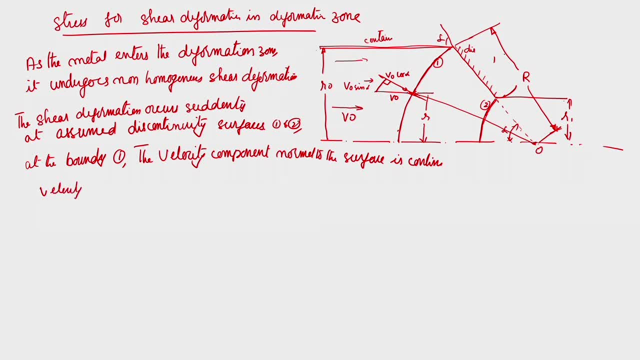 component: delta v, velocity discontinuity. delta v at the boundary is continuous, So this is parallel to the surface. so we can say that delta v is equal to v 0 sine alpha may be the equation twelve. So when, whenever it is a crossing this boundary, there is going. 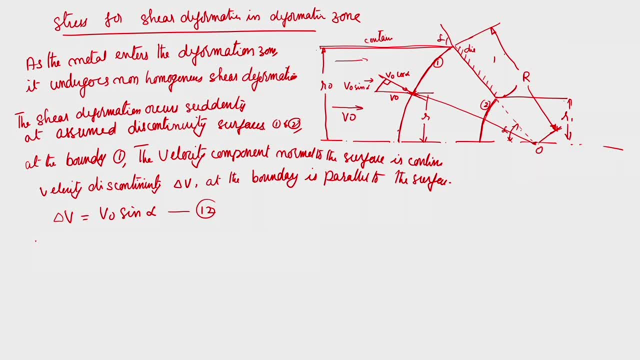 to be a sheer energy Right. Yes, the shear depending upon the velocity, shear energy rate at a given point, on the surface, at the entrance, at the entrance region. One is at the exit and another is at the entrance. We can say D We dot is equal to your tau of E mod emphaticitet value, rise to express heat. 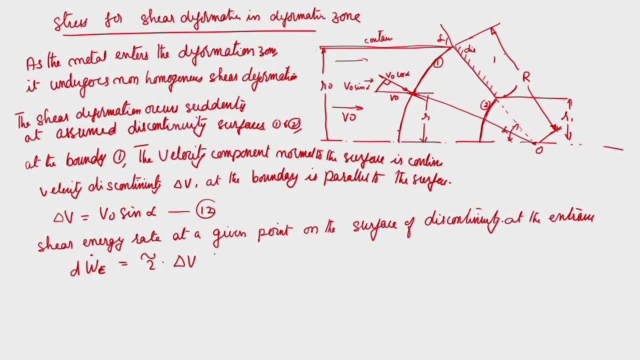 into delta v, the velocity discontinuity, into area, into d a, this is 13.. And we can see that toe is equal to m into sigma 0 by root 3, where for perfect sticking m is equal to 1 and d a is a surface element parallel to d v where the shear occurs. So we can from: 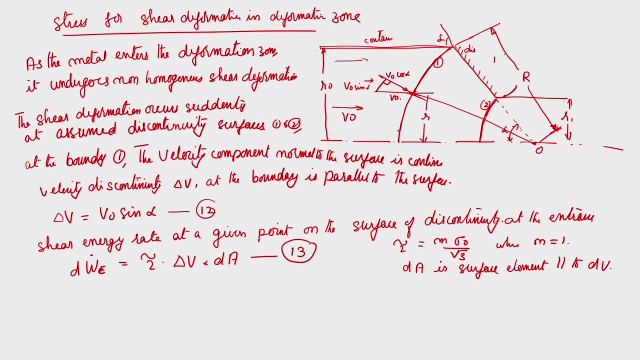 this geometry, this r is equal to say we can write r r naught. So we can write this geometric relationship: your r is equal to r naught by sin alpha and r is equal to r sin theta. this is alpha and if you take this as theta, So this relationship we can write So and d i is equal to 2 pi. 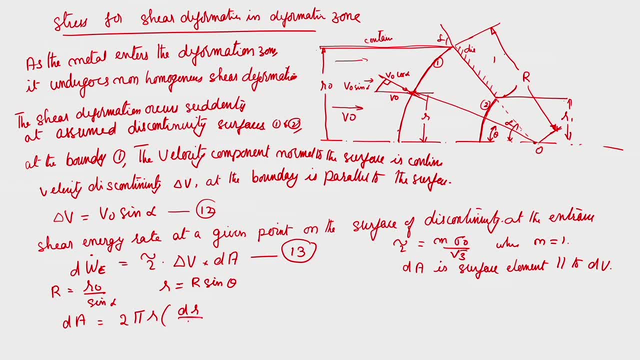 r into d? r by cos theta. we can write This relationship, so that is equal to 2 pi into r is equal to r sin theta, So you can say capital r sin theta into d? r by cos theta, cos theta. So we can write r cos theta d. 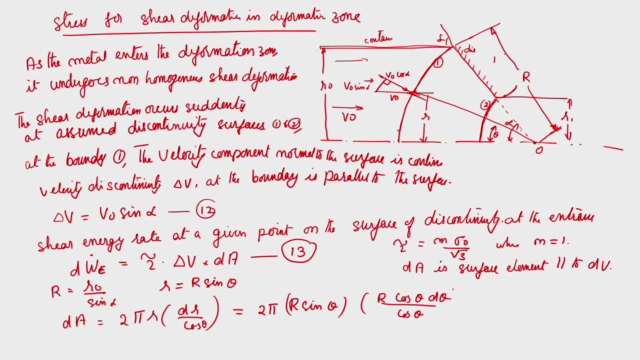 theta by cos theta, or that is equal to 2 pi into r is equal to r sin theta. So we can write from this: d a 2 pi r square sin theta d theta. So this is d a. So from this 12,. 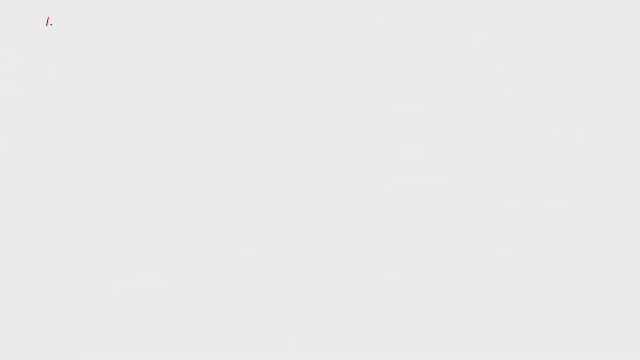 13, and 14, if you do a, if you substitute it in a, this equation from this, So we can just find it as d a into r sin theta, into d r, into d r square sine theta d theta. So, again, from this, click, the dimension that you can write: ok, Now, now that很好, we have. 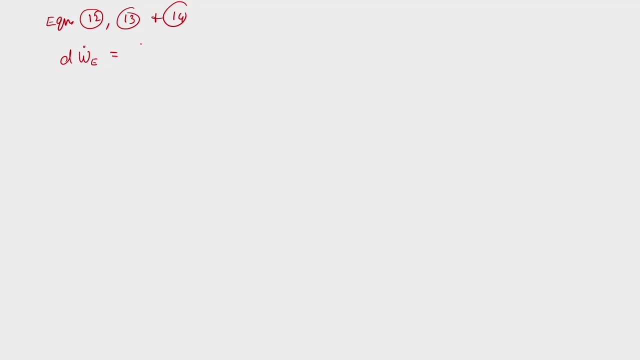 changed data We have, but also changed along. it is not due to the previous diagram. what w dot e is equal to, sigma 0 into root, 3 into v 0 sin theta into 2 pi r square, sin theta, d theta. So you integrate it, you will get the energy required. So that is w dot e is. 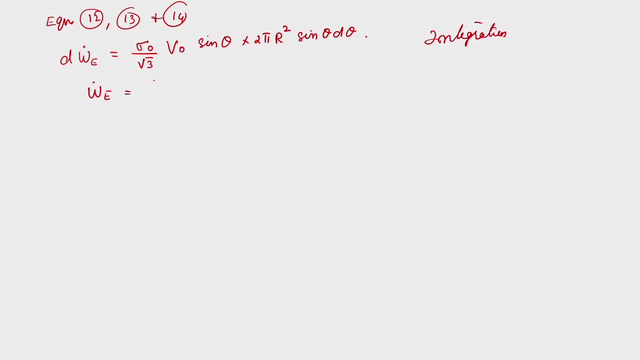 equal to strain energy right is equal to sigma 0 by root 3 into v, 0, into 2, pi r square, integral from sin theta, d theta, So that you will get it as sigma 0 by root 3 into v, 0, into pi r square, and simplifying. 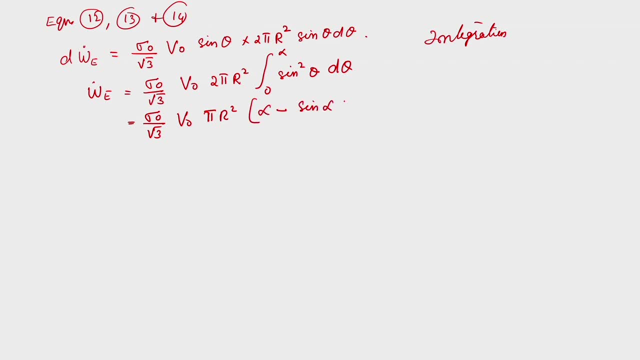 it you can get alpha minus sin alpha, cos alpha or w dot e is equal to v, 0 into 2 pi r square, sigma 0 by root, 3 into alpha by sin square alpha minus cot alpha, So that is 15.. Since 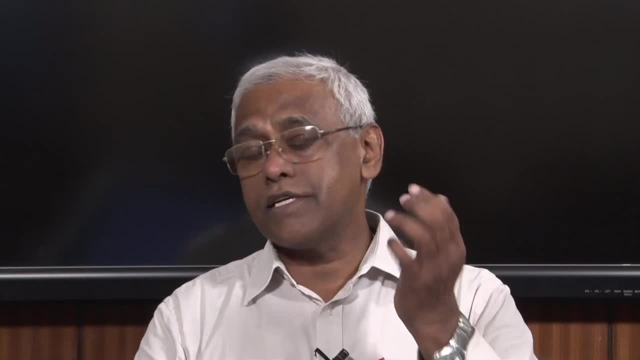 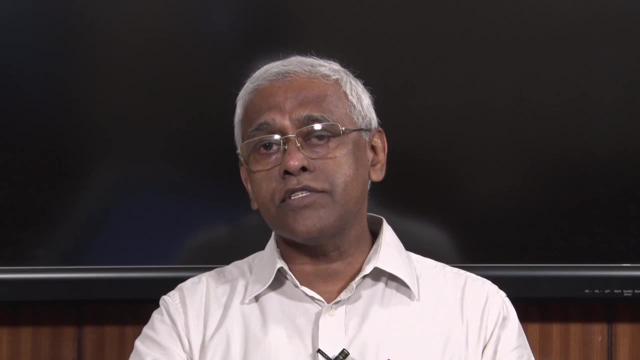 the shear occurs at the entrance and exit. at 2 region that shear discontinuity, velocity discontinuity is taking place. So shearing is taking place once it at the enter entry to the deformations on and at the other is at the exit to the deformation. So this is 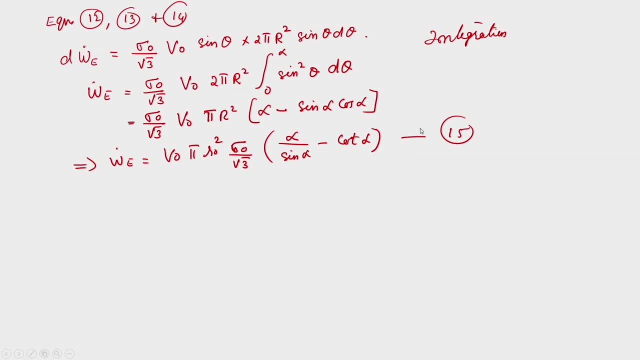 one and this is two, So these two regions are taking place. So since it is taking place twice, the total shear energy, total shear energy rate w dot t is equal to 2 w dot e, Since at entry and exit to the die. So we can say that the portion of extrusion load, the component 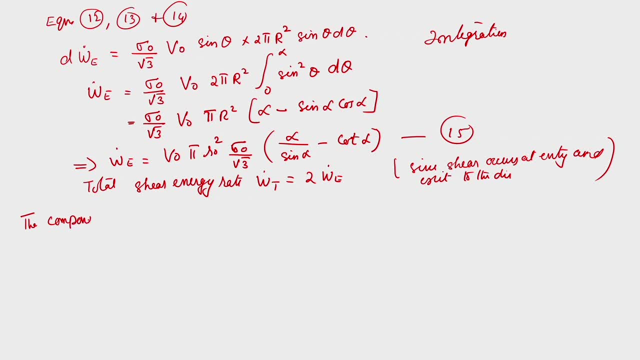 of extrusion load to overcome shear energy. overcome the shear. p d s is equal to w dot t by v. 0 is per unit volume. ok, So this is that. So we will get it as 2 pi r square into sigma 0 by root 3 into alpha.